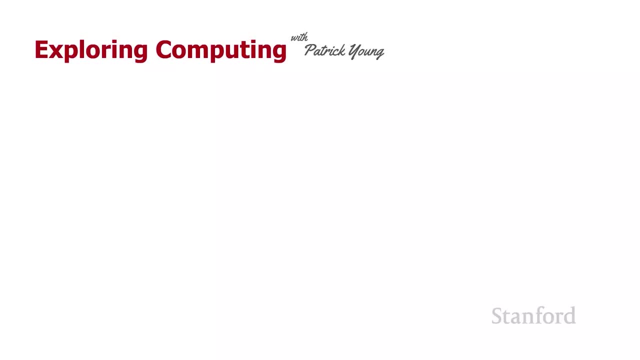 Welcome to Exploring Computing. Today's video is privacy, So I think the first thing we should talk about is: why is privacy different in the digital age? What makes privacy uniquely interesting in a networked digital world? So I think there's a number of changes. 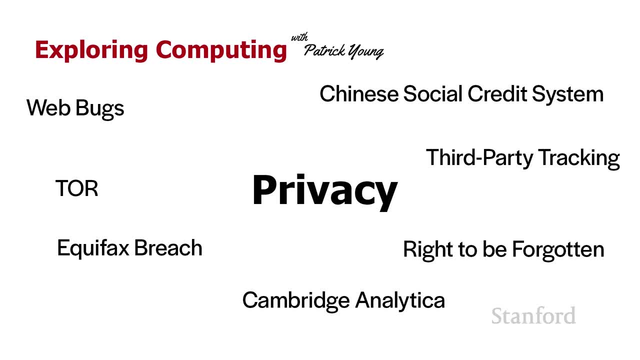 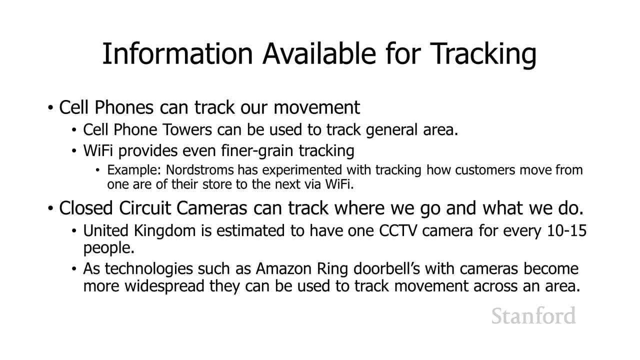 that have recently occurred that heavily impact privacy, And so let's talk about some of these. There's a lot more information available for tracking, So almost everybody has a cell phone at this point, and cell phones can track our movement. There's the obvious, which, as you move the cell phone around, 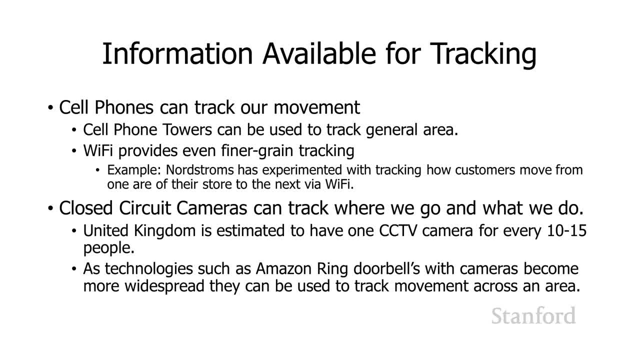 as you drive around the city, your cell phone is contacting different cell towers and that can be used to track your movements. But it actually turns out that you have much finer grain tracking than just the cell towers in many situations As your cell phone is moving around, 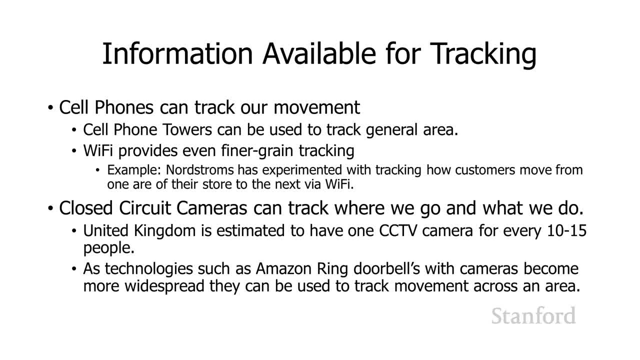 it is also contacting different Wi-Fi networks and different Wi-Fi routers as you move about an area And it turns out those can also be used to track your movements. So just to provide an example, Nordstrom says experiment with tracking how customers move from one part of their store to another by watching where cell 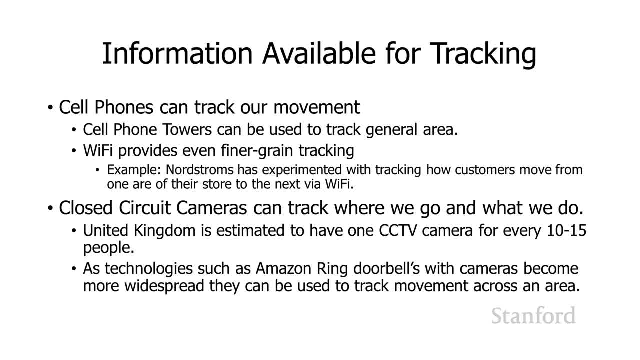 phones Try to connect to different networks as they move around store. Also, closed circuit television cameras are all over the place now and they can also be used to track where we go. The United Kingdom is estimated to have one closed circuit television for every 10 to 15 people. 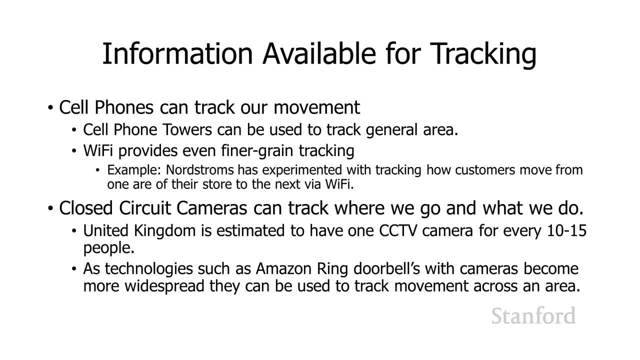 Technologies like Amazon's Ring doorbells with cameras also can be used to track movement, particularly once you have a relatively large number of these in an area. Then you can sort of put together the video coming from each of these different doorknobs. 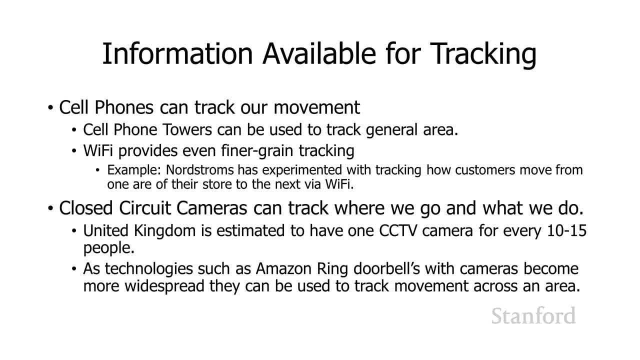 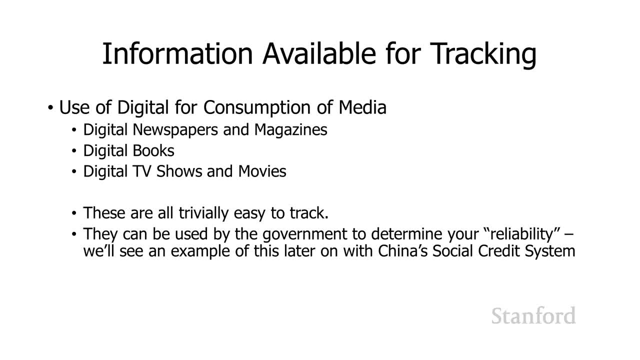 in order to track movement, And later on we'll be talking about how China is used in closed circuit television to track people as well. Also, as we move our consumption of media to digital devices, it makes it very simple to track our media consumption habits. 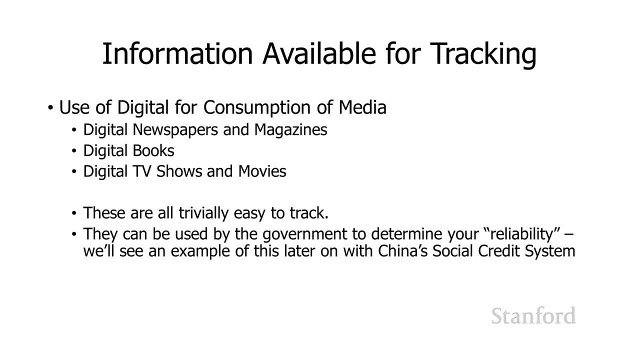 So digital newspapers and magazines, digital books, digital TV shows and movies, As long as you are not using physical medium, you are instead using digital medium. It's super simple to track everything that you're viewing, everything you're reading, everything you're watching. 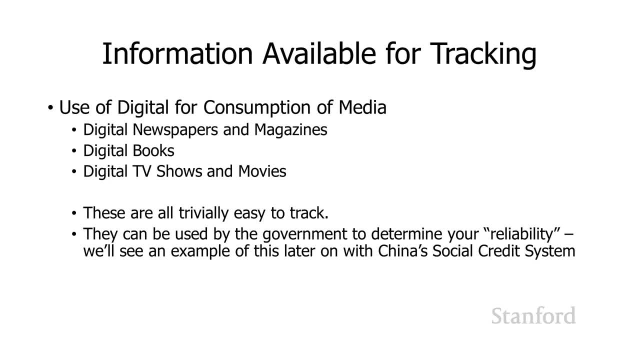 These can be used by the government to determine your reliability, And, in fact, we'll see an example a little bit later on how China may be using this for their social credit system, Being used to determine the reliability of their citizens and giving them rewards or punishments on that basis. 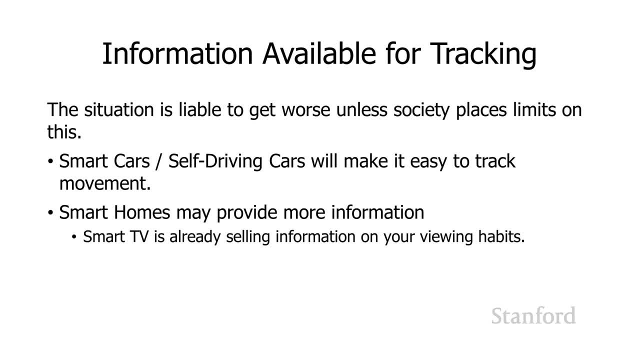 And I think the situation is liable to get worse, not better, As we move to smart cars which have some smart technology in them, and then we move to self-driving cars. it's going to be very easy to track your movements. Smart homes can provide information. 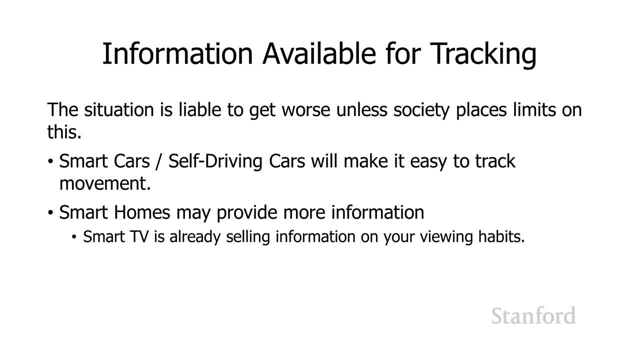 to whoever has access to them, on your activity And, in fact, smart TVs, which is pretty much most televisions that you would buy now- that have some sort of a- I suppose I can call it an- operating system. I think many of them are based on Android built into them. 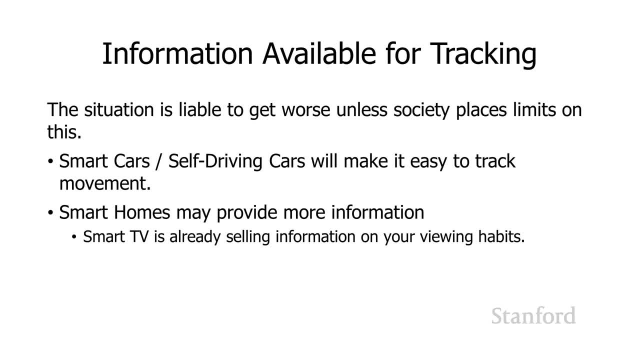 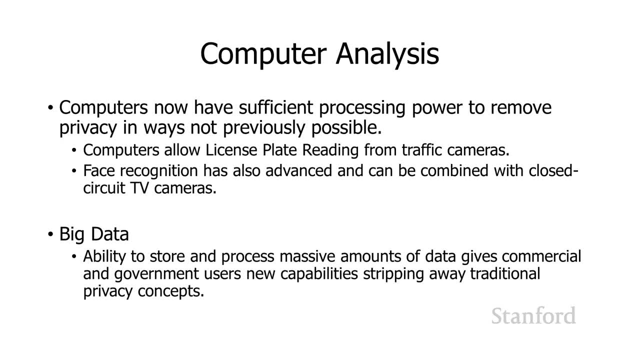 which allows you to put different applications on them and select different movies and watch different movies. Some of these companies are actually selling information about your viewing habits. So, in addition to having all this information, we now have sufficient processing power to really take advantage of it. 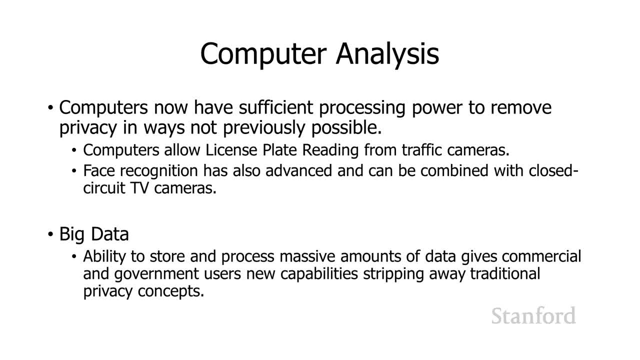 And this can also be combined with the ability to store a lot of information and then run processing after the fact on it. that gives us the ability to strip away things that were traditionally thought of as private. So previously, let's say, we were trying to track a particular vehicle across the city. 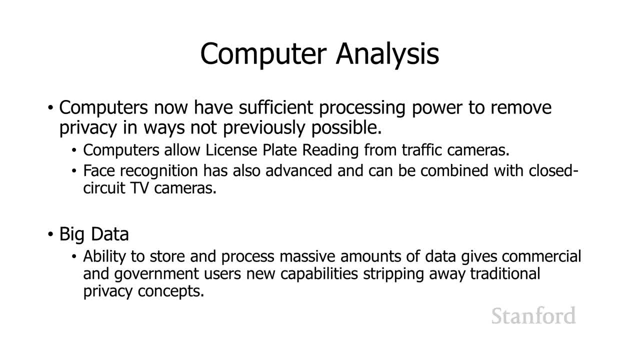 Maybe somebody had been kidnapped. We had some sort of a hostage situation And we were trying to track a particular vehicle across the city. Maybe somebody had been kidnapped. We had some sort of a hostage situation. Maybe somebody had been kidnapped. We had some sort of a hostage situation. 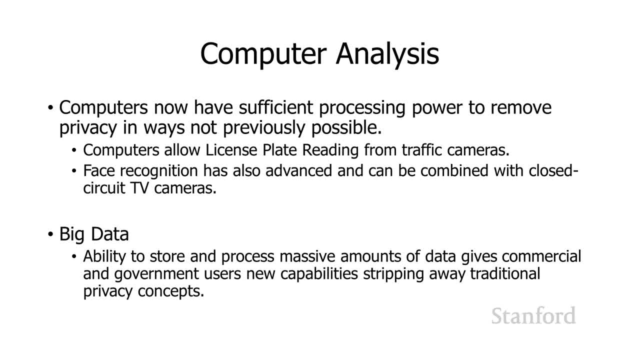 The police could use the closed circuit television cameras that are available in some streets that are used to track, to look at traffic patterns, And they could say, oh, we're gonna go ahead and watch the hostages vehicle travel across the city. and watch the hostages vehicle travel across the city. 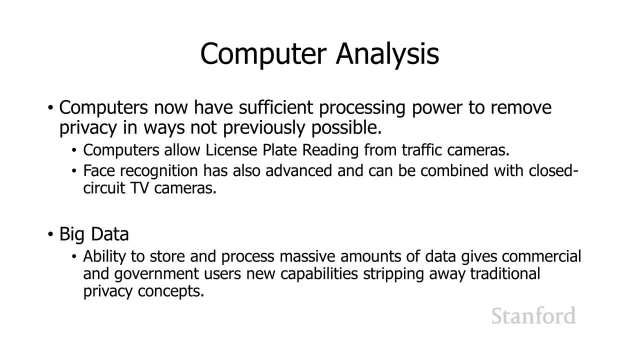 And so that's something they could do live before. but what we're able to do now, or the direction we're moving in as storage becomes cheaper and cheaper, is to store all the information from all the traffic cameras and start over and start over a period of time. 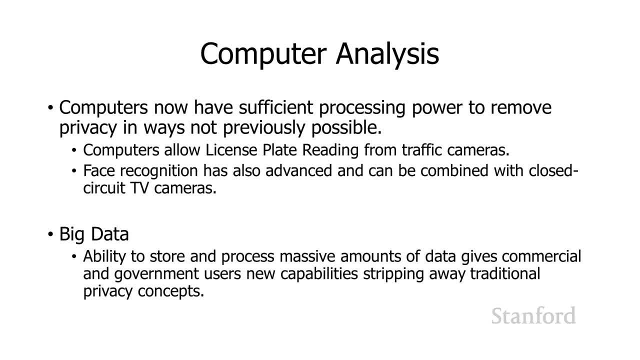 So the exact amount of time we would be able to save it would depend upon our storage capacity and how cheap storage gets. But you could certainly imagine a situation where you could store several days worth of traffic or at some point you may be able to store. 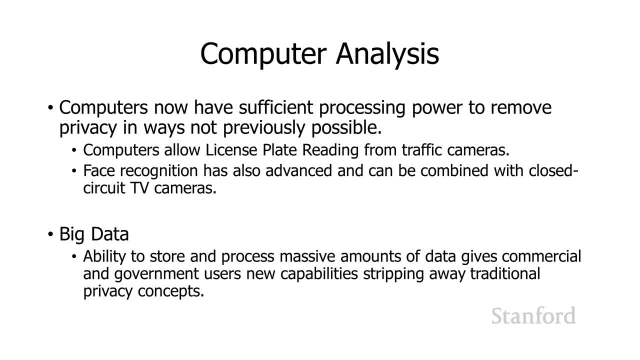 months worth of traffic and then process it later on. So maybe there's nothing going on right now. but then you're like, hey, so-and-so is. I think so-and-so is in a scandal. Let's go ahead and dig up the tapes from three months ago. 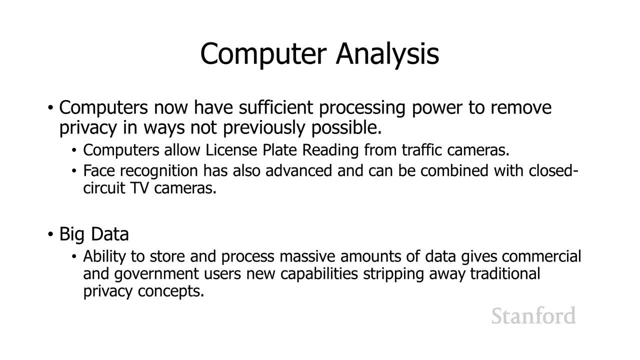 Here's his license plate number. Let's go ahead and see if we can search all of the data from all the traffic patterns to see if we can find his license plate number and then see what he's been up to. So I think the direction we're headed- 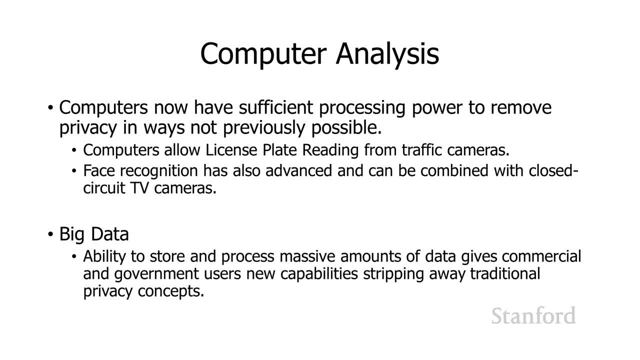 is potentially worrisome from a privacy standpoint is potentially worrisome from a privacy standpoint And this combination of all of these things- And this combination of all of these things- storing massive amounts of data and then being able to process it- 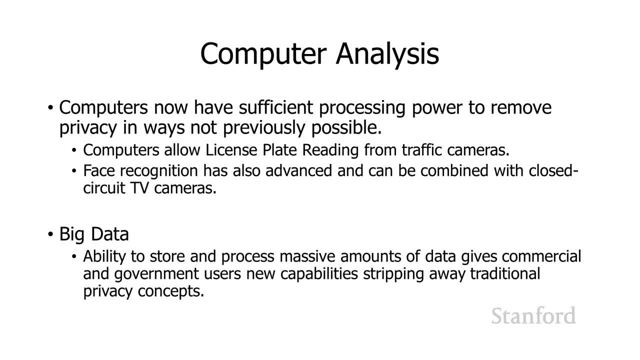 this is what sometimes referred to as big data, And it's something that's available for both commercial users and government users, And it's something that we may wanna think about like: do we wanna regulate this? What sort of society do we want? 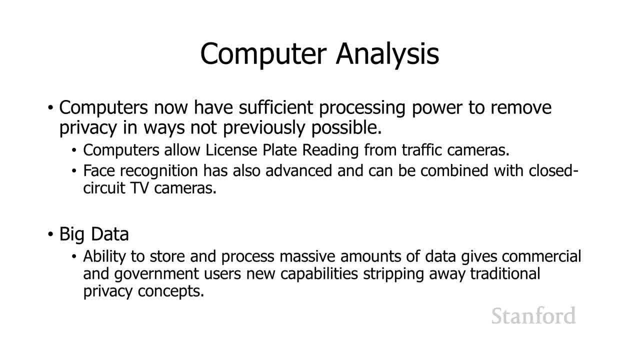 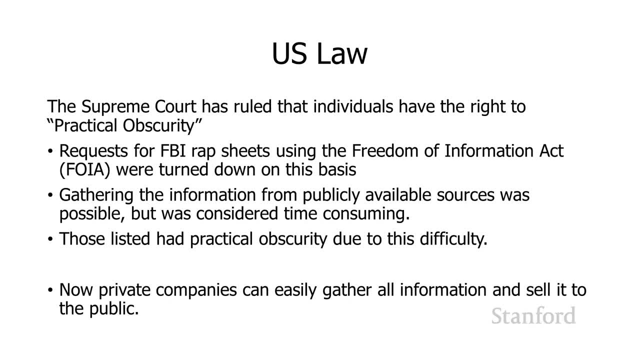 And we'll talk about this a little bit later on lecture, when we talk about both commercial issues with privacy and then government issues with privacy. Okay, so as far as US law goes, so it turns out that some of the protections afforded by US law are being eroded by our computing capabilities. 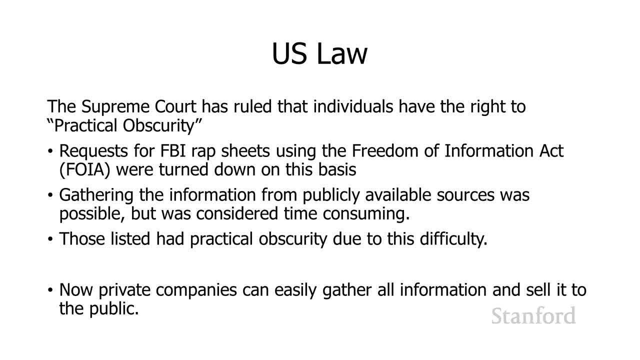 For example, the Supreme Court has ruled that individuals have the right to practical obscurity, And so the way this played out, or one example of how this played out, is that requests for FBI rap sheets using the Freedom of Information Act were turned down on the basis of the need for practical obscurity. 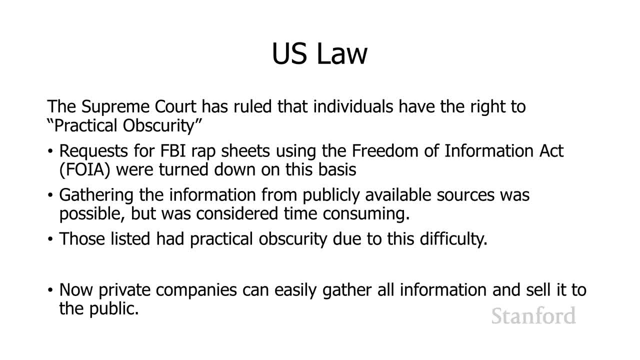 And while that information was publicly available, the idea is that somebody would have to go through and gather all of that publicly available information And that was a time consuming thing. So those listed had practical obscurity because of the difficulty of tracking down all the information. 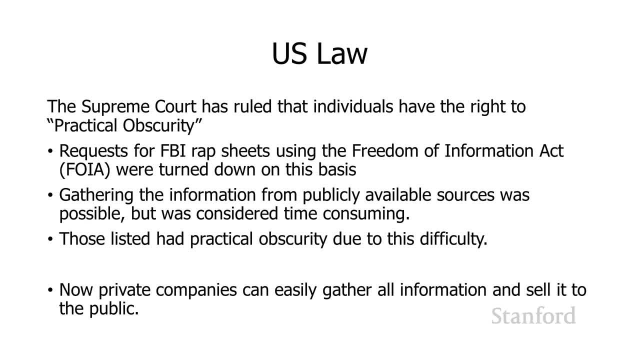 But of course, now it's trivially easy to track down information. In fact, companies gather this information. You may have seen their advertisers on the web like: hey, do you wanna look up what your high school significant other was doing? Look them up, find out where they live now. 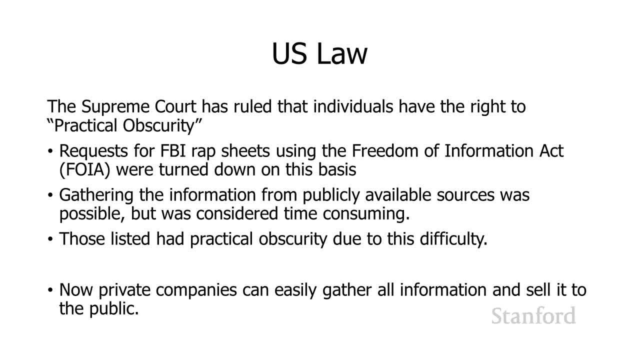 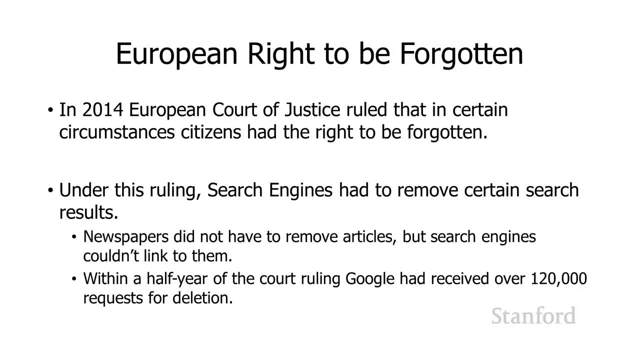 find out what their income is, find out if they're married. So the practical obscurity is largely gone because of computing power. The European community is probably doing the best job of being active, trying to protect the privacy of their citizens. There's been several things that they've done. 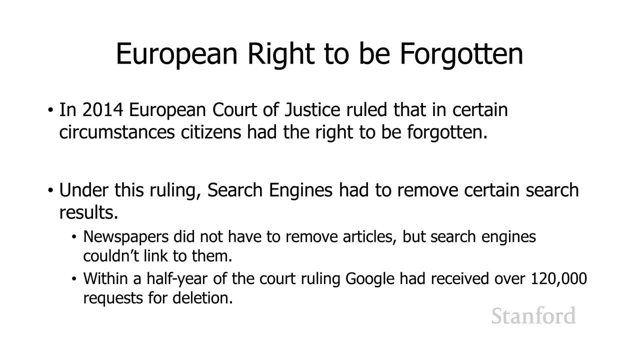 One thing that they've done is that, in 2014,, the European Court of Justice ruled that in certain circumstances, its citizens had the right to be forgotten, And under this ruling, search engines had to remove certain search results. So if a newspaper had an article, 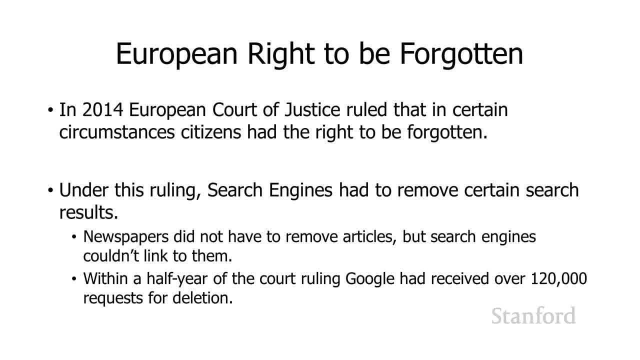 that they had written previously. they were still allowed to leave that up on their website, but search engines couldn't directly link to those articles. Within a half year of the court ruling on the right to be forgotten, Google had received over 120,000 requests. 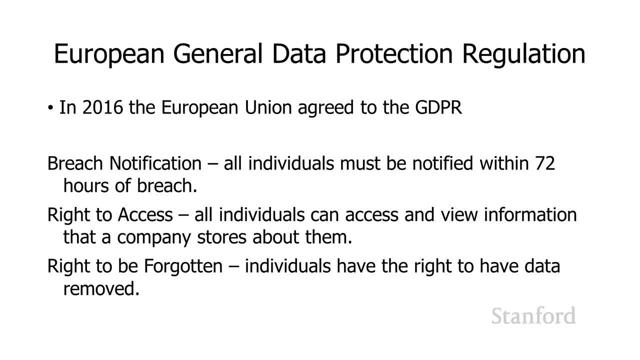 for deletion of information. Another move that the European community has made is the European General Data Protection Regulation, And this was agreed upon in 2016 and took place two years later. You will most notice this because of the annoying popups that you're constantly getting. 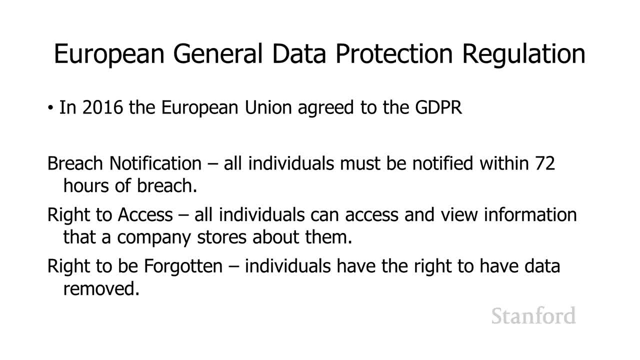 whenever you visit a website saying: are you okay, star information? I mean. it turns out that California has also made similar moves very recently, So- you may be getting some additional populace because of California's new laws. So what does the General Data Protection Regulation actually? 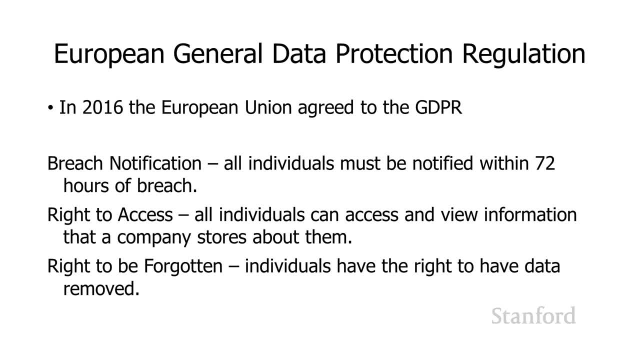 do. Well, here are the key things that the GDPR requires. If a company is storing somebody's information and is breached, individuals must be notified within 72 hours of a breach. It's not unusual without this law. it's not unusual for a company to not even tell people. 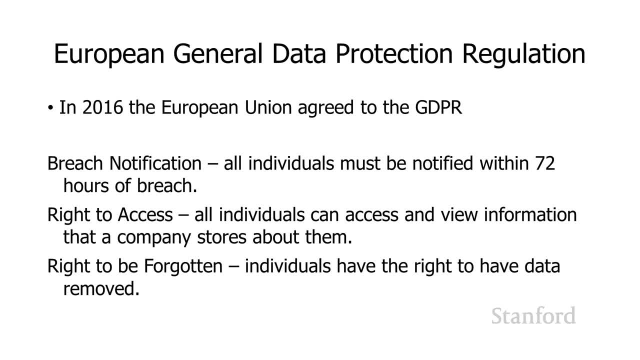 that their data is out there or to wait as long as possible, In spite of the fact that people knowing their data is out there might be an important thing for those people to be able to protect themselves. GDPR requires all individuals whose information has been leaked to be notified within 72 hours. 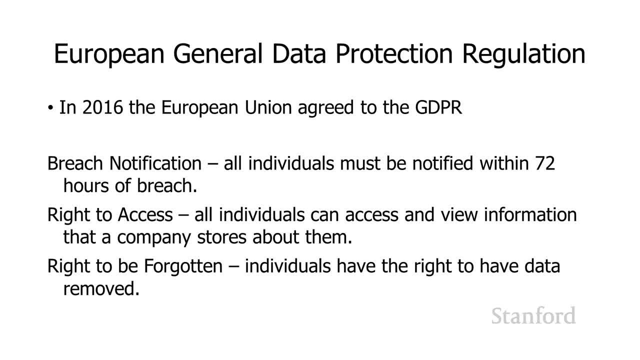 Individuals also have the right to access the information that the company is storing about them. They have the right to have data removed about them And they have the right to have data removed about them And they have the right to have data removed about them. 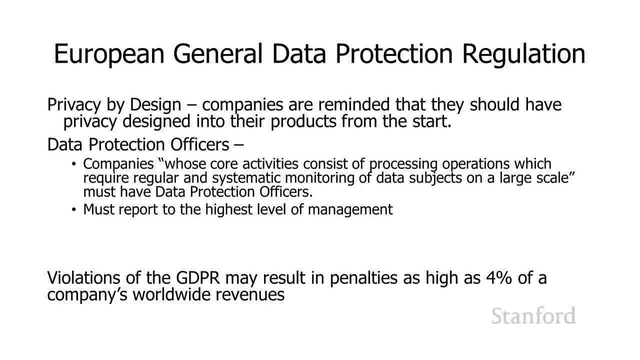 And companies are reminded that they should have privacy designed into their products from the start. In addition, companies that fit into certain characteristics must have data protection officers, And those data protection officers must report to the highest levels of management And they're responsible for making sure. 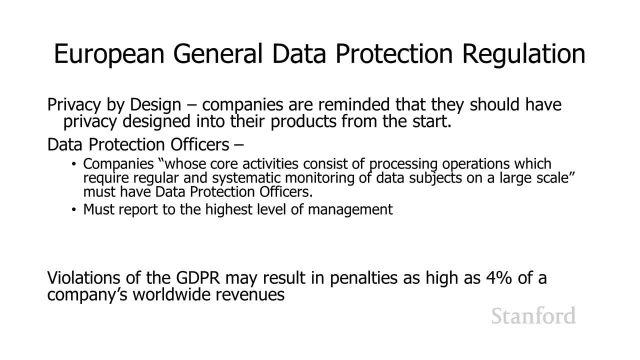 that the data is properly protected. Violations of the GDPR do have some teeth, And they may require Penalties as high as 4% of a company's worldwide revenues. All right, let's take a look at commercial use of data. 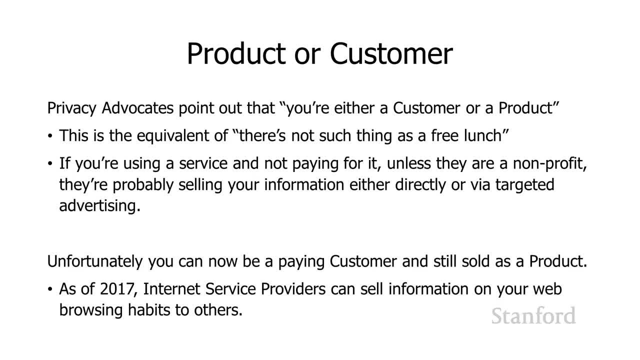 So one thing that privacy advocates sometimes talk about is this concept of you are either a customer or a product, And so this is basically saying there's no such thing as a free launch If you are using a product and you are not paying for it. 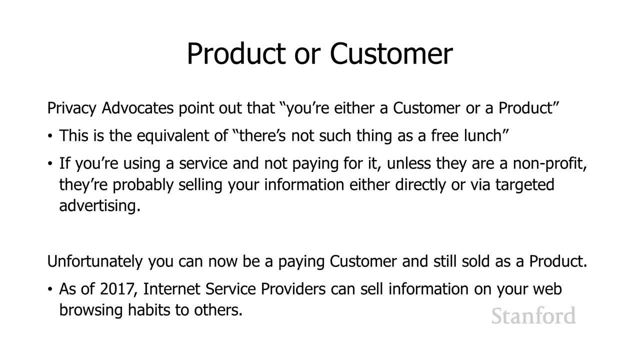 and you are not getting that service from a company, from a nonprofit or perhaps the government, then the company that you are getting that service from needs to be making their money somehow. If you're paying for it, well great, That's how they're making their money. 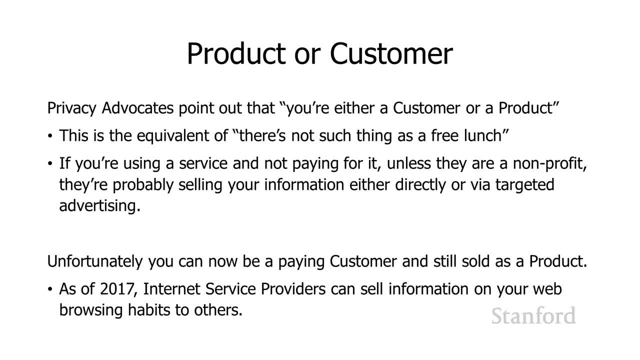 If you're not paying for it, then probably they're making money by selling either access to you or information about you. So either directly, they're taking information about you and selling it directly, Or They are showing targeted advertising to you And unfortunately it's now possible for you. 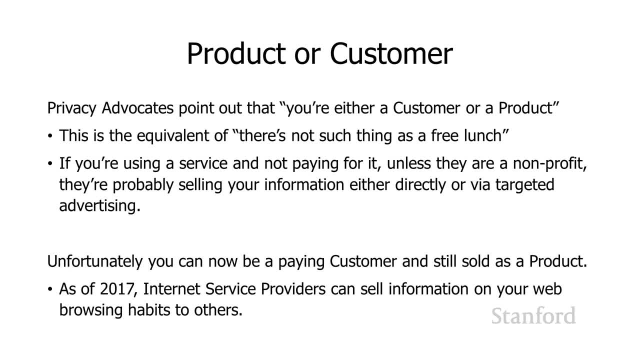 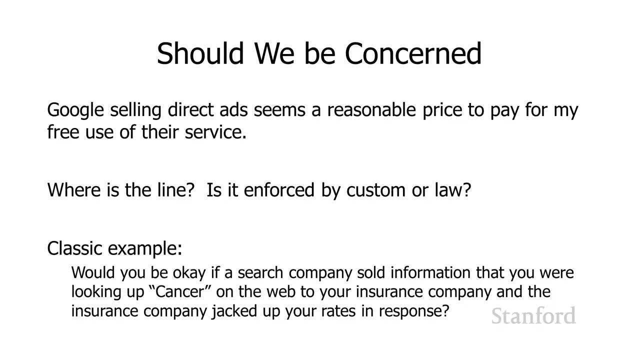 to both be a customer and also be a product. So, just as an example, as of 2017, internet service providers can now sell information on your web browsing habits to others, even though you are actually paying them for your internet service. So should we be concerned? 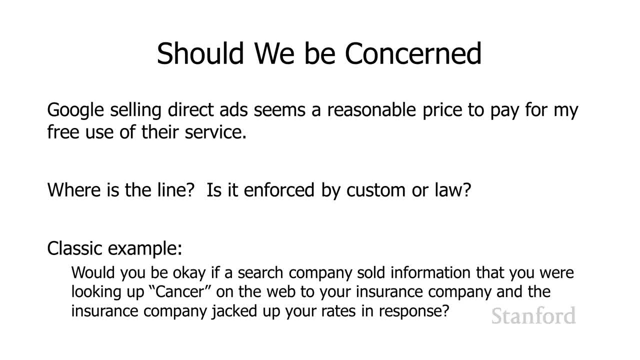 So one thing to be thinking is: Hey, I use Google or I use Bing or I use, I guess, DuckDuckGo- I can't think of any other services offhand- as my search engine, And obviously they have to pay the bill. 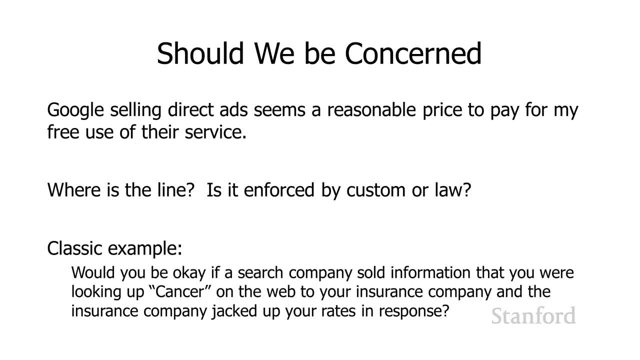 So seeing targeted advertisements because I'm able to use Google for free, that seems like a reasonable thing. But the thing to be concerned about is where is the line? And is that line enforced by custom or is it enforced by the law? And to give you sort of a classic scenario, 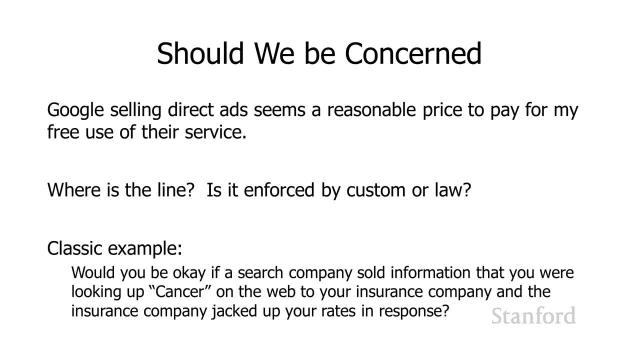 that privacy advocates have put out there. if I am searching websites looking for things about cancer, perhaps I have a friend who has cancer, or a parent has cancer, or I have cancer. there's no way they know. But is it OK for the search engine? 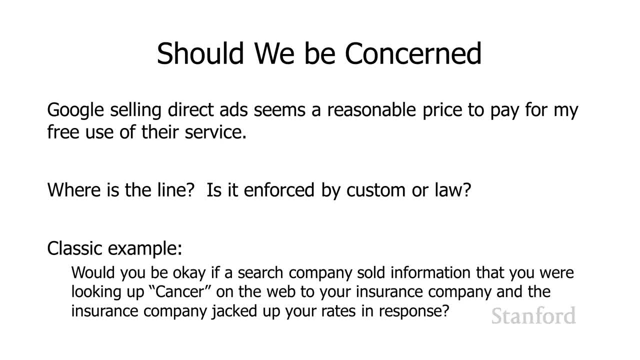 to take the information that I am searching- searching for cancer- turn around and sell that information to my insurance provider and for my insurance provider to jack up my rates on the theory that I might actually have cancer. Are we OK with that? And if we're not OK with that, how is it going to be enforced? 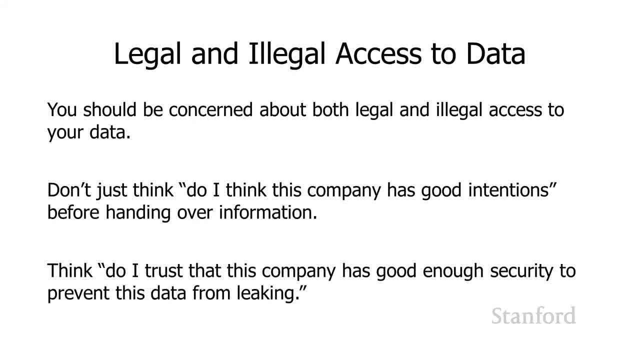 All right. another thing that you should be thinking about when you are entering information that you think of as private onto a website or providing it to a company is: OK. OK, Is this something that it would be legal for them to share with people? 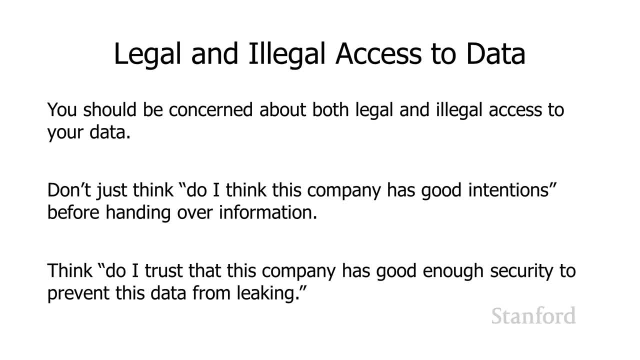 But also, is it possible that someone might illegally gain access to this information? So, in addition to thinking, do I think this company has good intentions, you should also be thinking: do I trust this company has good enough security that this information isn't going to actually leak? 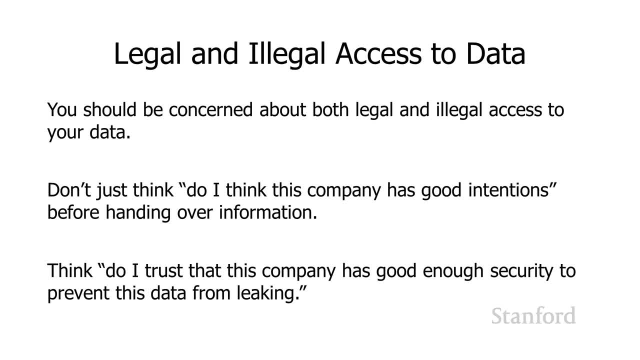 that they're not going to get hacked in spite of whatever good intentions they might have, And so let's take a look at a couple examples where maybe people shouldn't have trusted these companies with our information. All right, so one of them is Equifax. 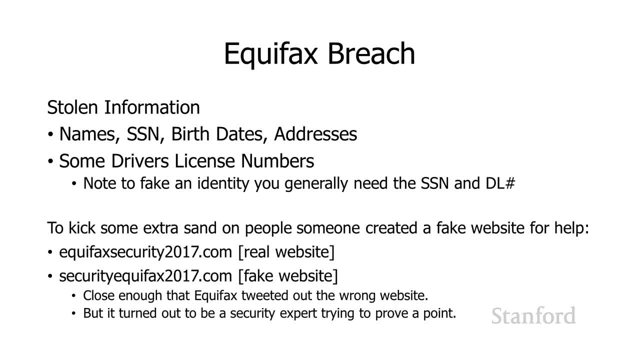 So Equifax is a credit agency. It's one of those companies that keeps track of what we do in the financial world and with our credit cards and whether or not we're credit worthy, OK. And so they got breached And a lot of people had their names, their social security. 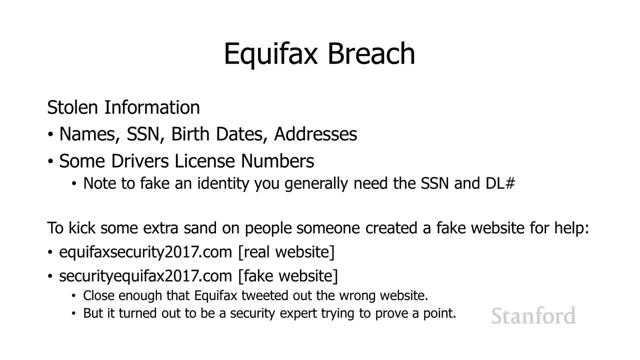 numbers, their birthdates and their addresses stolen in this breach And, in addition, some of them had their driver's license numbers stolen And it turns out that if you have a social security number and a driver's license, you create fake identities. 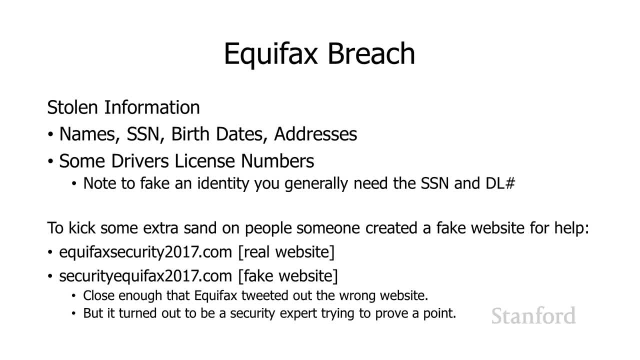 and create credit card accounts for people. So that combination right there is super dangerous. And just to kick some action, I'm going to throw some extra sand on to the people whose information was breached. Someone created a fake help website. There was a real website for help called EquifaxSecurity2017.com. 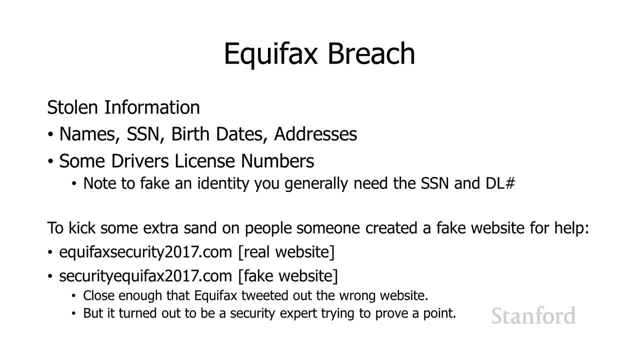 Somebody created one called SecurityEquifax2017.com, And it was close enough that Equifax accidentally tweeted the wrong website out on their Twitter account. But the good news is, in this case, the fake website was created to kind of make a point. 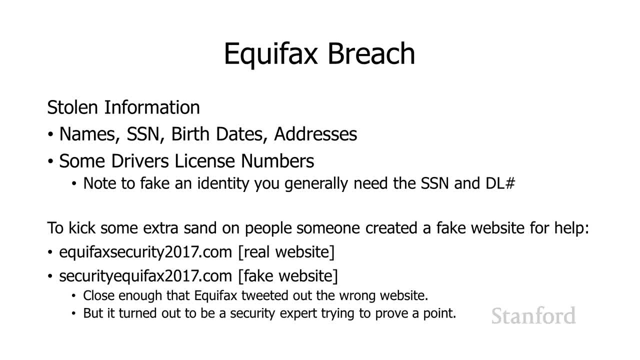 The other thing that's a little bit odd about the Equifax breach is: none of us are customers of Equifax. We don't really agree for our information to be up there. I mean there might be something, some fine print in the credit card, credit cards we sign up for. 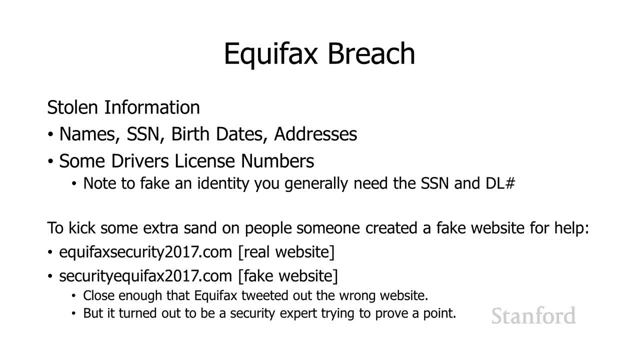 or maybe the banks we work for. that says they're able to pass the information on Equifax, But none of us are directly customers of Equifax, And yet they had all this information and that information was all lost. OK, here's another famous example: Ashley Madison. 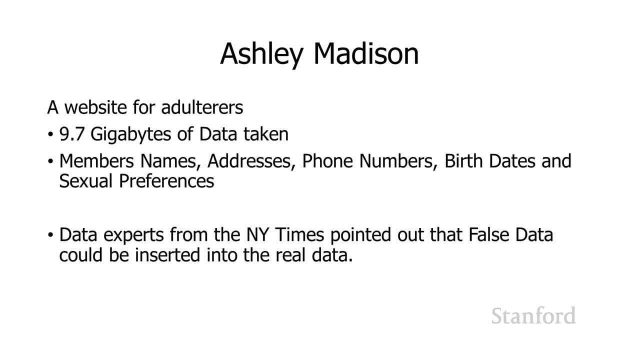 If you're not familiar with Ashley Madison, that's probably a good thing. Ashley Madison was a dating website for adulterers and they got hacked And 9.7 gigabytes of data was taken, including members' names, addresses, phone numbers. 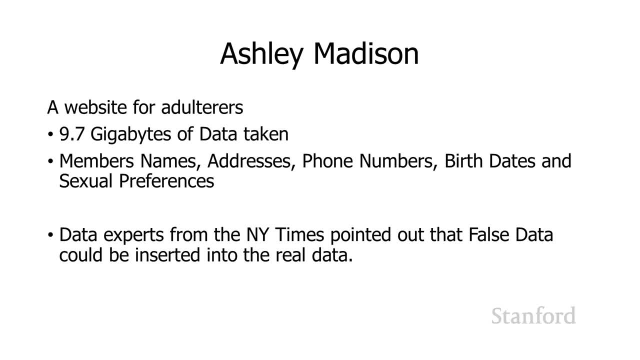 birth dates and sexual preferences. One thing that the New York Times pointed out was that, when this information was released, it was entirely possible for the hackers to insert some fake data into it. So yeah, Anyway, so people trusted Ashley Madison with their information. 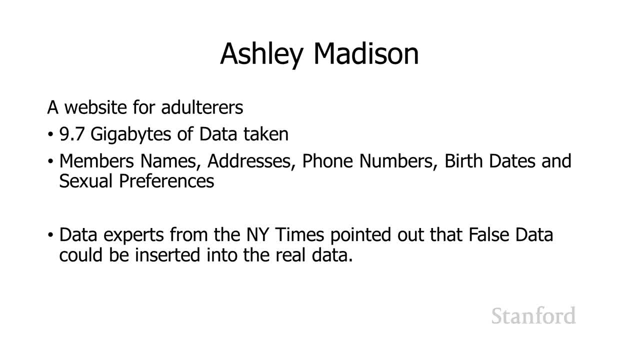 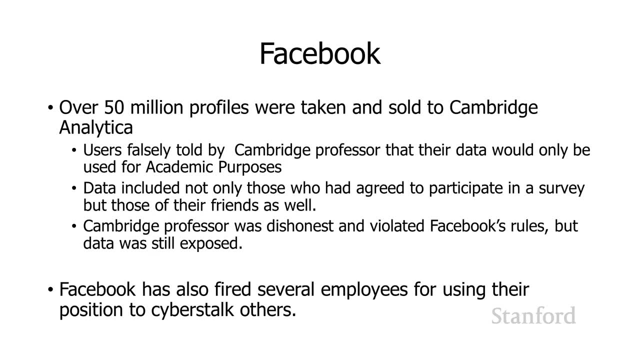 They shouldn't have. Perhaps Ashley Madison had good intentions, but they did not have good computer security, All right. so our next example is Facebook. Over 50 million profiles on Facebook were taken And sold to Cambridge Analytica. Users were falsely told by a Cambridge professor. 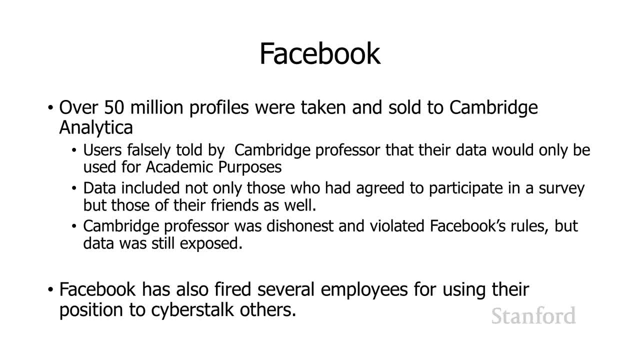 that their data would only be used for academic purposes. But not only was the data for those people who thought it was only going to be used for academic purposes taken, but it also turns out that the professor involved was able to access information on their friends as well. 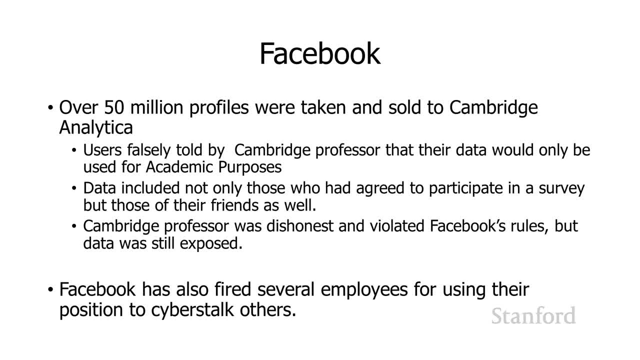 And so this is a little bit different than the previous one. It's a little bit different than the previous examples, because it wasn't that the company got hacked, but it was rather that they were working with somebody and that somebody violated the terms of agreement. 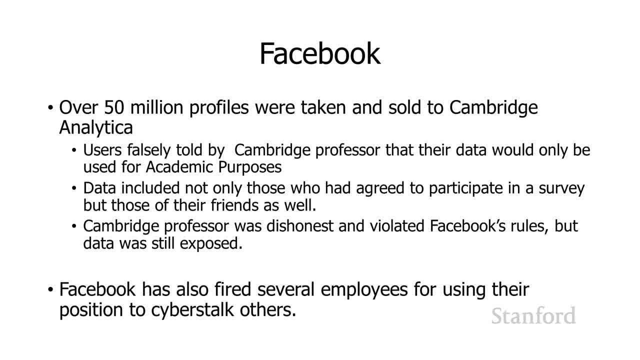 and did something that was dishonest, But nevertheless the people involved had their information taken and stolen and sold to a third party. Facebook was not technically hacked, but people sort of fell for what turned out to be kind of sort of a scam Where the person had intentions to do something untrustworthy. 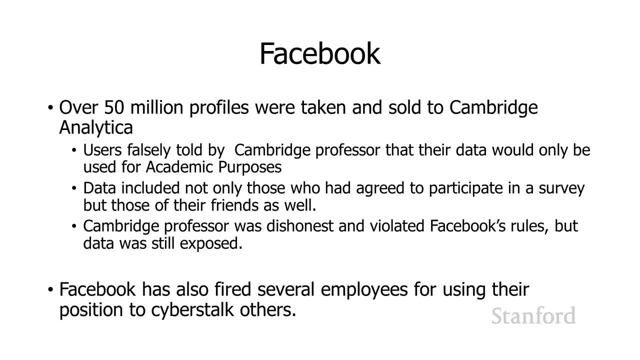 You could argue that this is arguably a case of social engineering. In addition, Facebook has had several occasions where they've had to fire employees because those employees were cyber-stalking people taking advantage of their position at Facebook to cyber-stalk. So these are both reminders that if you put information up, 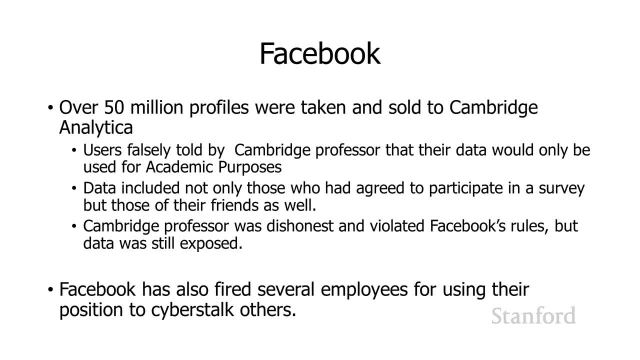 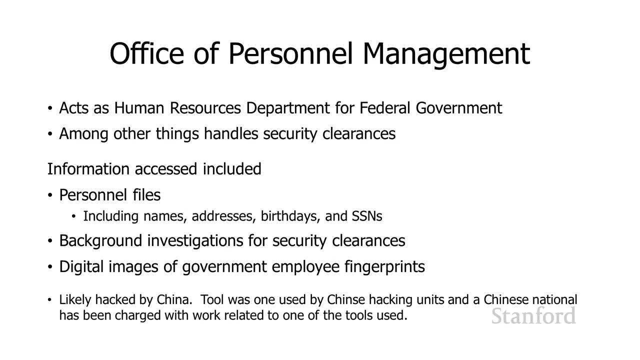 there, even if the company has good intentions, not to share that information in ways that you might not want it shared, it is possible that bad things will happen and the information will leak anyway. All right, our last example is the Office of Personnel Management. 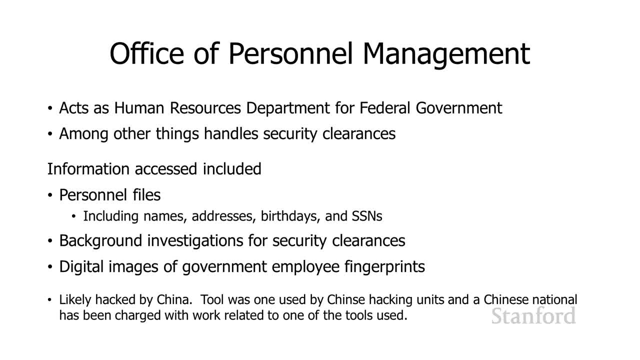 The Office of Personnel Management acts as a human resource department for the federal government And, among other things, it handles security clearances. And they got hacked. Information access included personnel files with names, addresses, birthdates and social security numbers. Probably more troublesome, it included background. 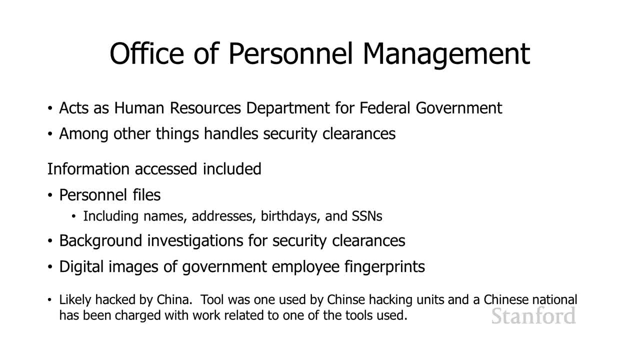 investigations for security clearances, which includes things like: have you done drugs? Are there things that you've done that might lead to you being blackmailed? So these are all the sorts of things that might go into a background investigation And it's going to be stored on their computers, which 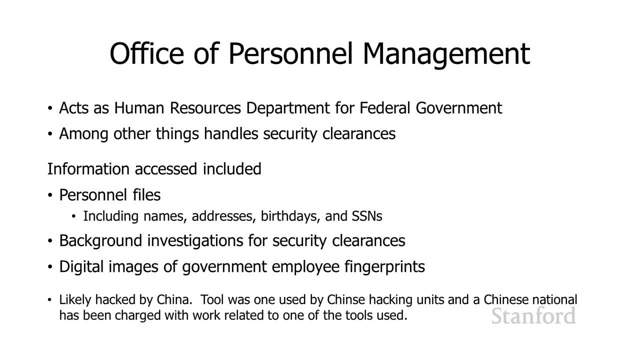 got hacked. Good job, guys, All right. In addition, digital images of fingerprints for government employees were also stolen. Now, as to who did the hack, it was probably China. The tool used is associated with Chinese hackers And, in fact, the Chinese national. 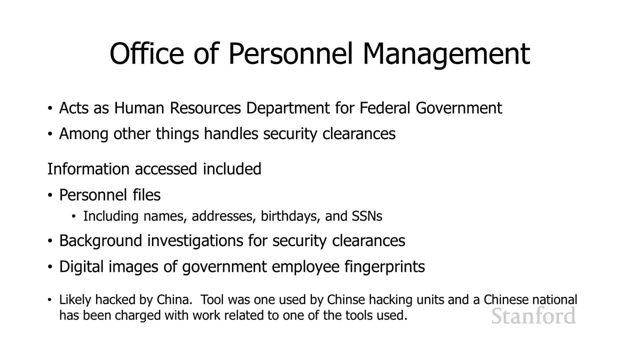 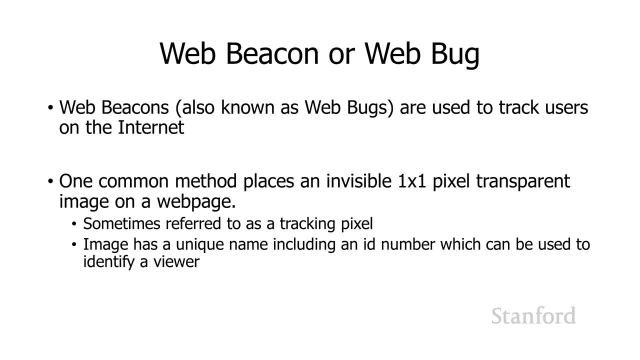 has been charged with work related to one of the tools used in the Office of Personnel Management. hack here. All right, let's move on to tools and techniques related to privacy. So one technique that is used to breach privacy is something called a web beacon or a web bug. 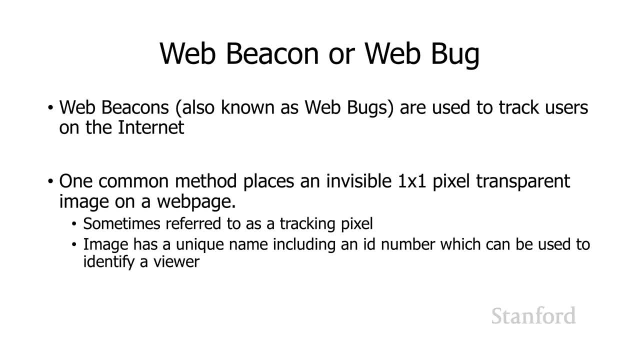 So these are used to track users on the internet, And you guys can figure out how these work because you know how HTML works and you know how HTTP works now. So, essentially, what a web bug or a web beacon is is, it's a one by one image that appears on a web page. 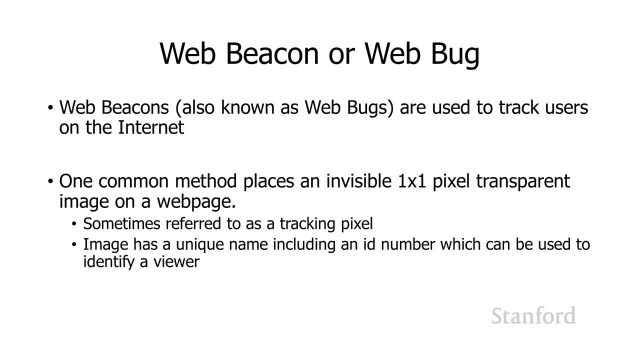 It's transparent, so people don't actually notice that it's there, And this is sometimes referred to as a tracking page. OK, It's a tracking pixel, And the idea here is this: tracking pixel has a unique ID number which identifies the specific individual who this web page has been served up to. 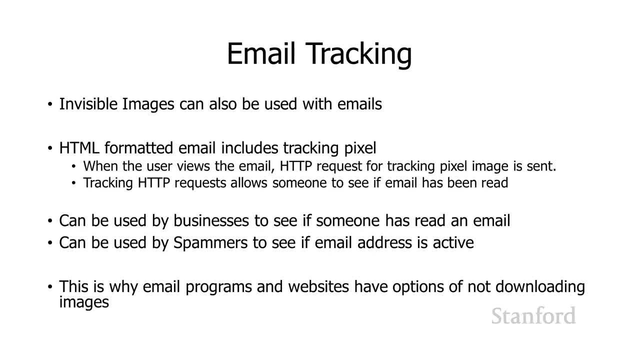 And this can be used for several different purposes. So one thing it can be used for is email tracking. So if you've got an invisible image on a HTML mail file, what happens is when somebody opens up that mail file, the HTML file has that IMG. 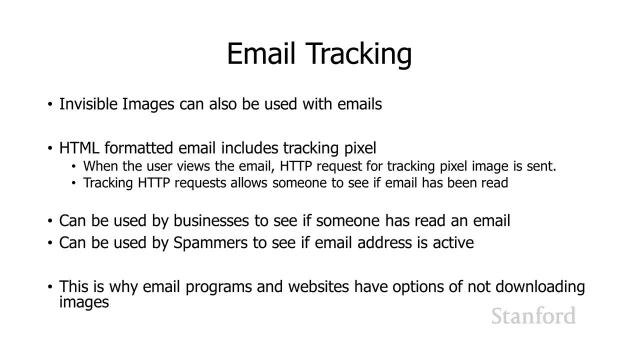 SRC equals. It's got the name, has that unique ID number for this particular email And when the server gets hit by a request for that invisible tracking pixel image, it says: oh, the person with that ID number just opened up the email message. 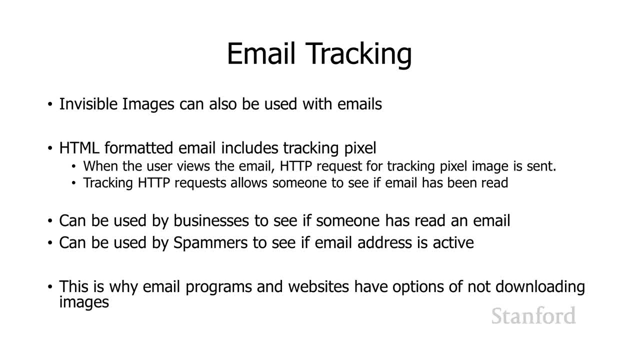 That's why I'm getting a request for that particular tracking image. It can be used by businesses to see if somebody's read a particular email. It can also be used by spammers to see if an email address is active. So the spammers send out a bunch of emails in HTML. 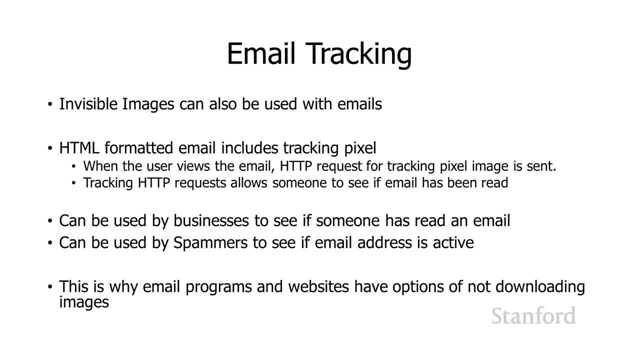 And all of the emails are exactly the same, except for the tracking beacon. And so there's going to be an IMG, SRC, equals. and then there's going to be a unique ID number- dot. JPEG, or a unique ID number- dot. PNG. And now what's going to happen is when you go ahead, 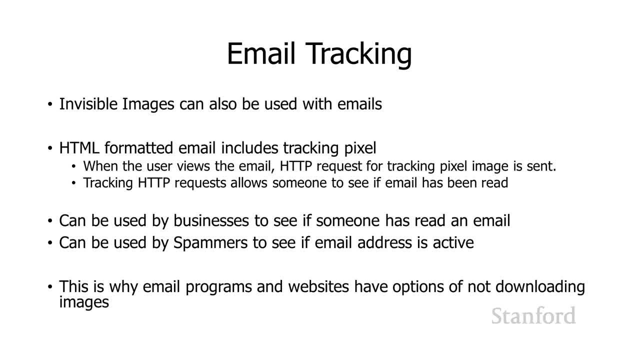 and receive that email. if you're, email is set up to display images, your web browser is going to, or your email program is going to send an HTTP request to wherever that tracking beacon is coming from And it's going to send a request for the particular image. 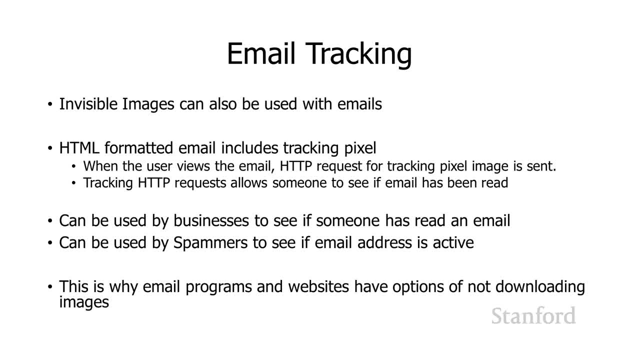 file with that unique ID number that only you received an email message, And then the server on the other side is going to see that that specific ID number was requested And it'll be able to match it up with the original email message that was sent. 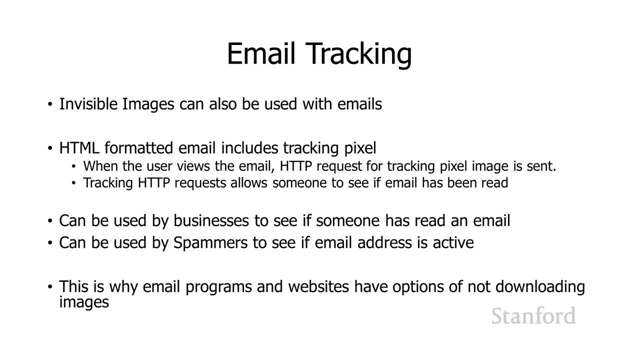 And you may have noticed that a lot of email programs have an option to not display images until you specifically say: oh, I trust the sender, Go ahead and display the image now. And this is the main reason why they do that: to prevent tracking of email. 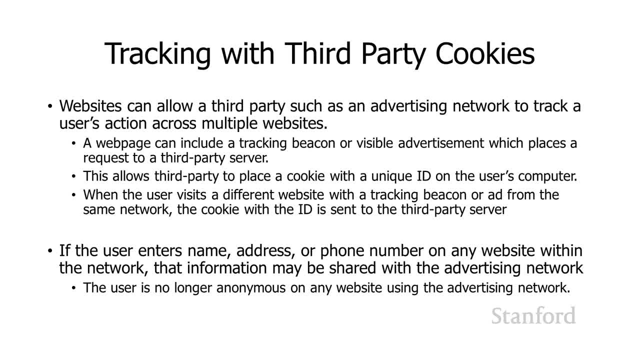 These can also be used to track people's movements across the internet with third party cookies, And so when we're talking about a third party, what we're talking about is the first two parties are you and the website that you're visiting. So that's party one and party two. 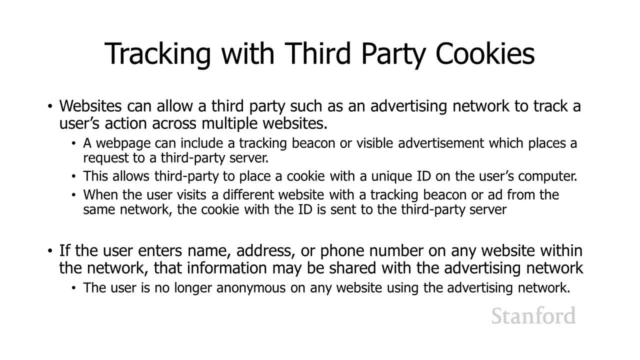 And party three is some other party. So the idea here is that a website can allow a third party, such as an advertising network, to track a user's actions across multiple websites, And this can be either done with these tracking pixels that we were just talking about. 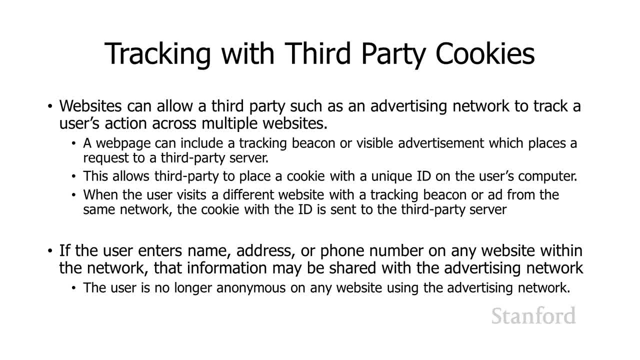 Or for these invisible, one by one pixel images, Or they might actually be done with the visible advertisements. But what happens here is that when you visit a web page that is participating in this third party network with cookies, what will happen is, in addition to the regular contents of that web page. 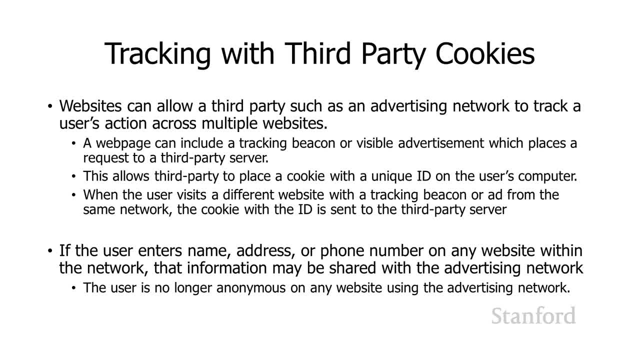 you will also. the HTML file will also reference either that tracking pixel web beacon image or it will reference an actual advertisement that shows up on the web page. Either way, it is requesting that web beacon or that image file not from their servers, but from the third party servers. 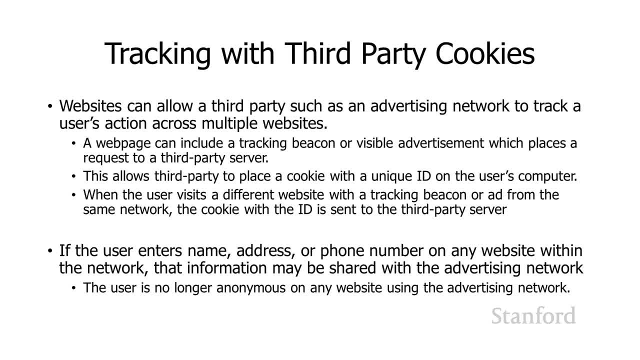 When you make that request to the third party servers, what happens is that third party sends that image, whether it's the tracking beacon or an actual advertising, And in addition, it places a cookie on your web browser. So cookies store is a technique used. 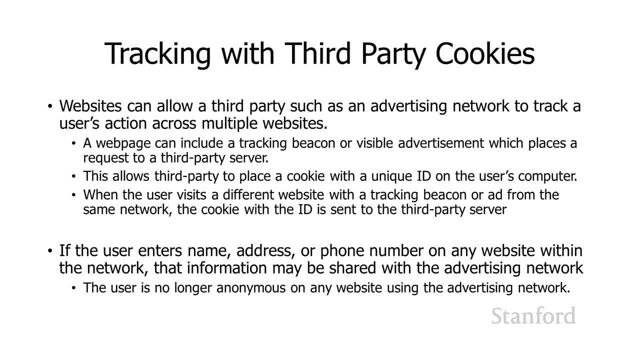 to store small amounts of information in your web browser that can be sent back to the website the next time you visit it. So let's say you go to Amazon. Amazon is going to put a little bit of information in your web browser such that the next time you visit Amazon, 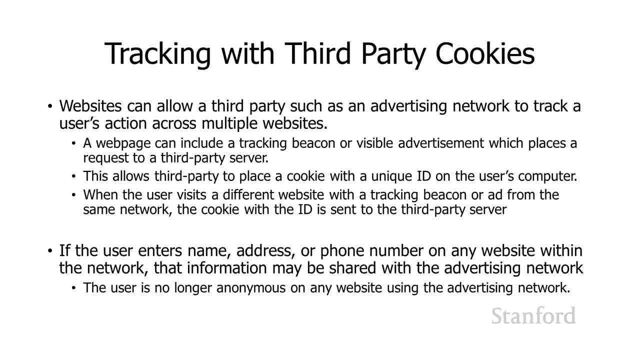 your web browser is going to send that information back to Amazon, And that's how Amazon actually knows who you are the next time you visit. Similarly, if you've got subscriptions to things, so like I have a subscription to New York Times, The New York Times keeps track of me. 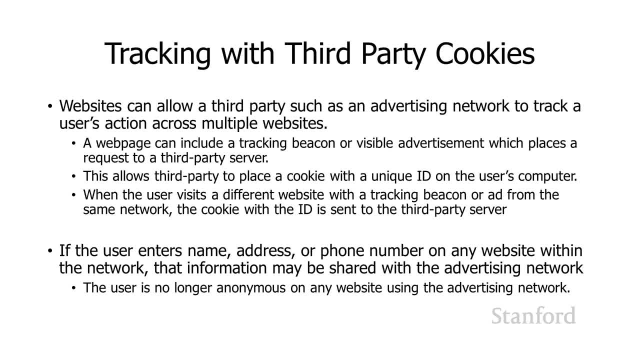 by putting this little cookie on my web browser, And the next time I visit the New York Times, my web browser sends that cookie back to New York Times when I visit it and says: oh, that's Patrick, He has academic access to New York Times, so he's fine. 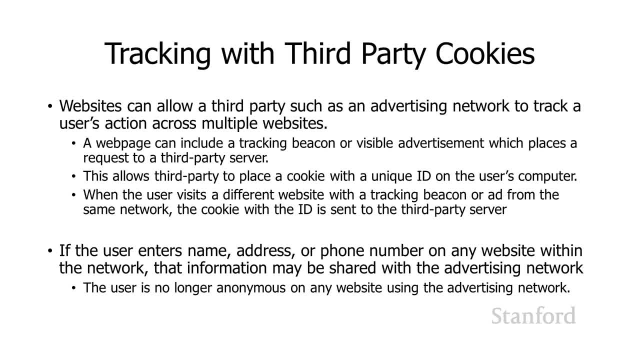 Yeah, That's fine. So the idea here is these third-party networks, because the HTML files have references to images from these third-party servers. the third-party servers are able to send you tracking information and put this cookie information into your web browser. 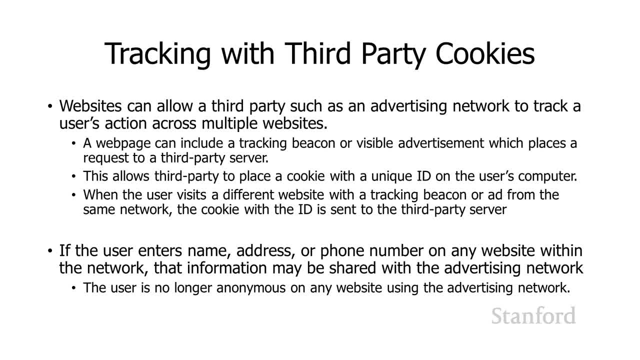 Now, when you move to a different website, if that website is also serving up images again, whether they're these invisible web beacons or they're visible advertisements, when that request to that third-party, that advertising server, comes up, the third-party cookie. 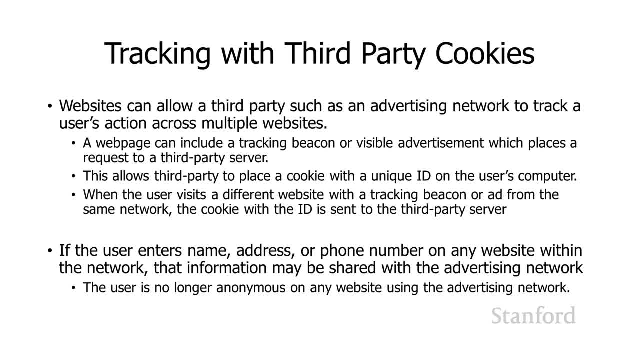 that they had put in previously is also going to get sent to them. So they'll be like: oh, this is the same user. I saw this user on this other website. I'm now seeing them in this website And they can build up a picture of all the different sorts. 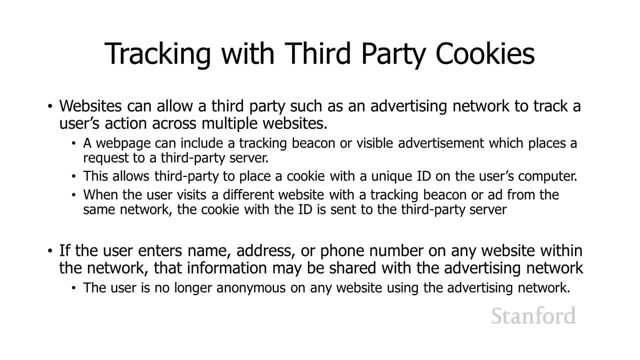 of websites that you visit. As long as you are visiting different websites on that tracking network, they will be able to send you, and they will be able to build up, all the information about what your web browsing habits are and form a profile for you. 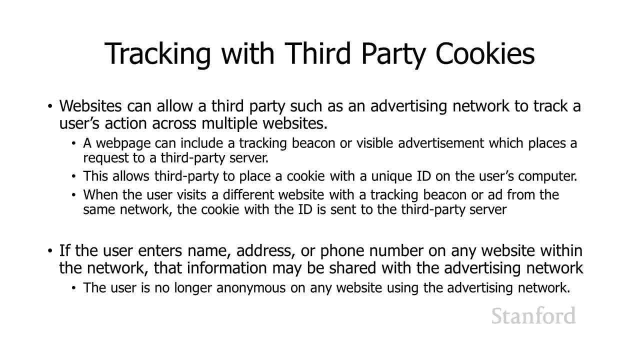 Now, depending on what they want to do. if you were to actually enter information into one of these network websites, like, let's say, these advertisers are showing up on a store web page, or maybe the store was working in conjunction with the advertising network? 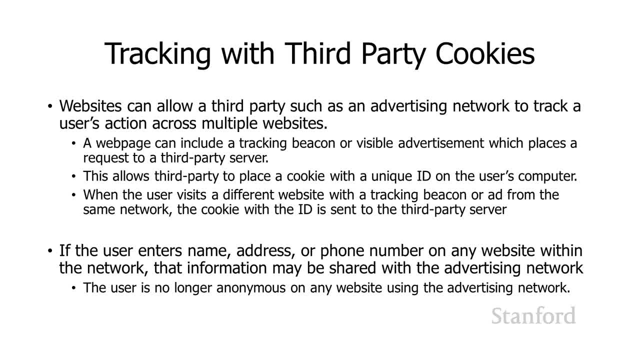 even though the store wasn't actually displaying images and I enter in my name And phone number and other information. that information can be used in conjunction with the advertising network If that website chooses to pass that information onto the advertising network. the advertising network. 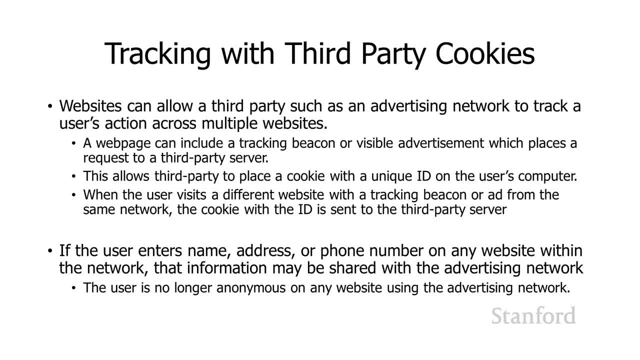 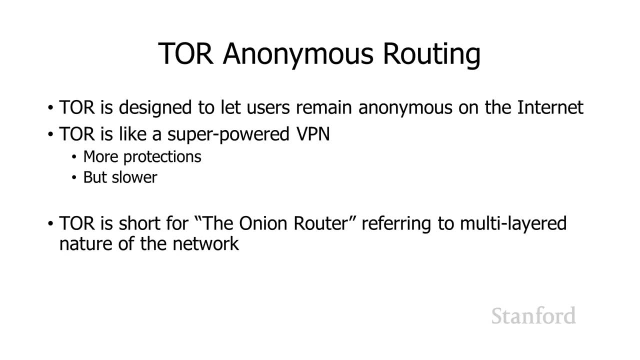 not only has an idea of what my web browsing habits are, but potentially they could have my name, address and phone number and whatever other information I entered into the main website that was working in conjunction with the tracking website, All right, So this doesn't sound very good. 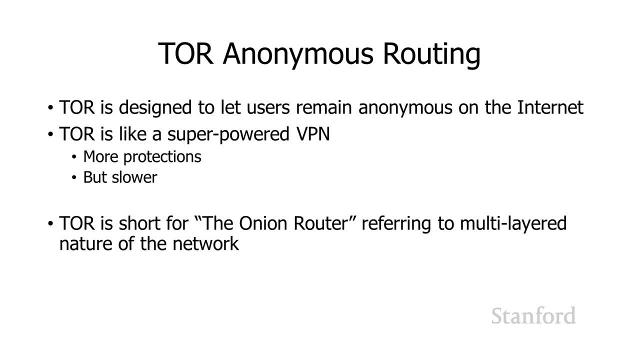 What can we do to protect our privacy? Well, last lecture we talked a little about VPNs, virtual private networks, and how they do provide some privacy. If you want to go further, there's something called Tor. Tor is a special routing system that. 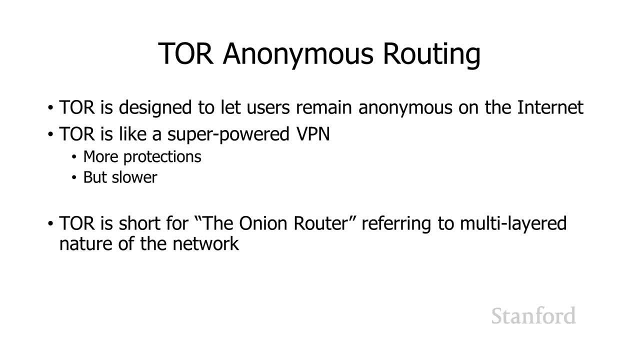 is designed to let users remain anonymous on the internet. You can kind of think of it like a super-powered VPN with more protection, but it's much slower. Tor actually stands for the Onion Router, which refers to the multi-layered nature of the network it uses. 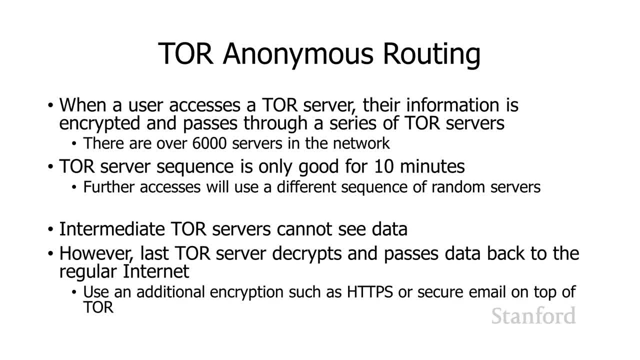 When a user accesses a Tor server, their information is encrypted and passes through a series of Tor servers- And there are over 6,000 servers in the network- And so when you go ahead and access something through Tor, what's going to happen is you are going to get a special. 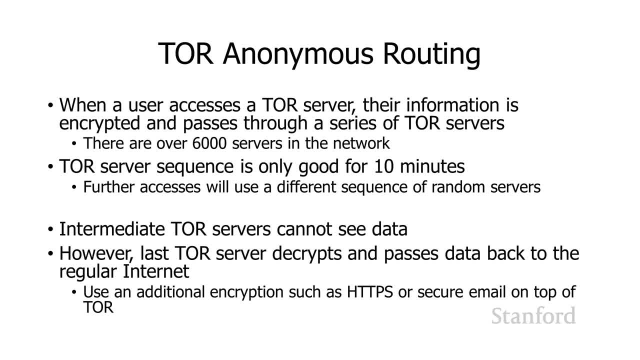 sequence through the Tor network, where your information is going to get passed from one Tor server to another Tor server to another Tor server And when the information comes back, it should follow the same route. That information, that routing information, is only good for 10 minutes. 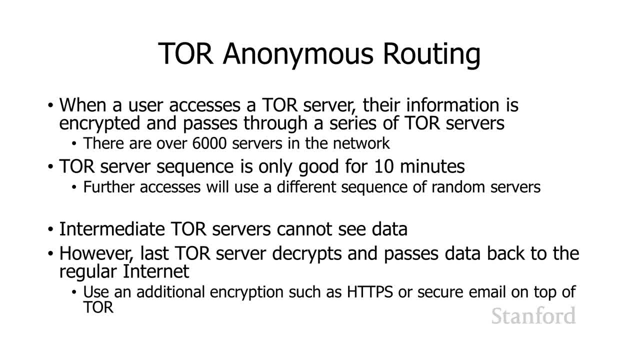 And if you make another access after 10 minutes you're going to get a different sequence of random servers. The intermediate Tor servers cannot see what the data is But ultimately, in order for you to be able to access it, to access the regular internet, ultimately on the far end, 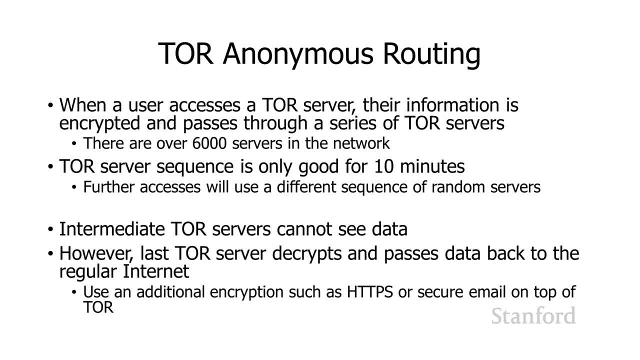 that information is going to have to be decrypted And the destination for your request needs to be discovered, And so the last Tor server is going to be able to have some idea of the information that you've sent. And so, if you want your information, 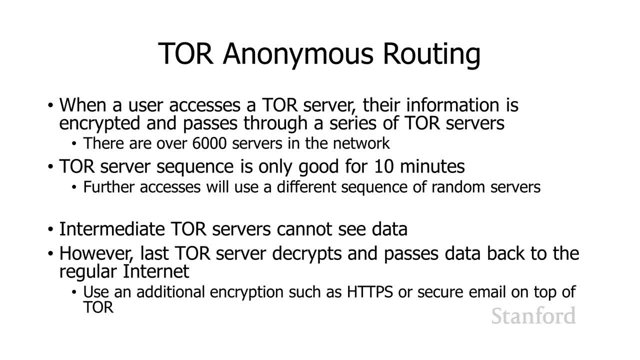 to be completely hidden from the Tor server. you need to use encryption on top of just using Tor, So you could use something like HTTPS or secure email. Just be aware that by using Tor by itself, you are not fully encrypting your data. 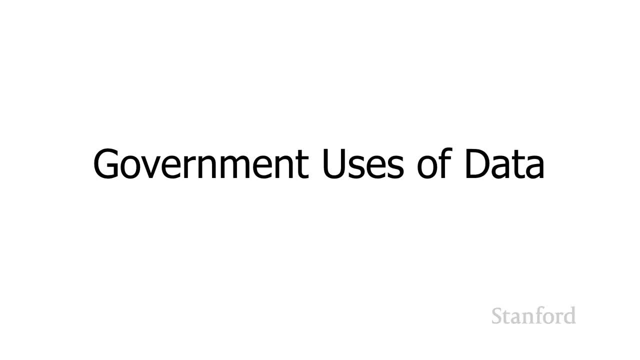 All right, let's talk about government uses of data and government concerns with privacy. So one thing that I've often joked about in class is that I really don't care if the NSA can read my emails. So the basic idea is: well, I'm going. 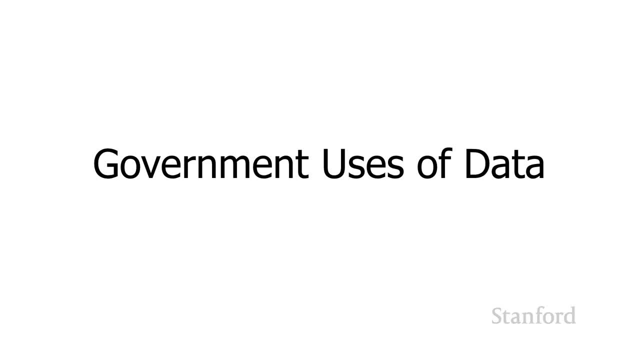 to be able to protect myself against random hackers. But if the NSA wants to break into my accounts, I am not claiming to have such good security that the NSA is not going to be able to break my stuff and read the emails I'm sending to my students. 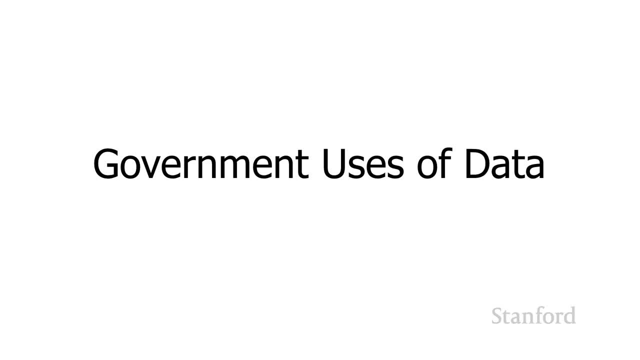 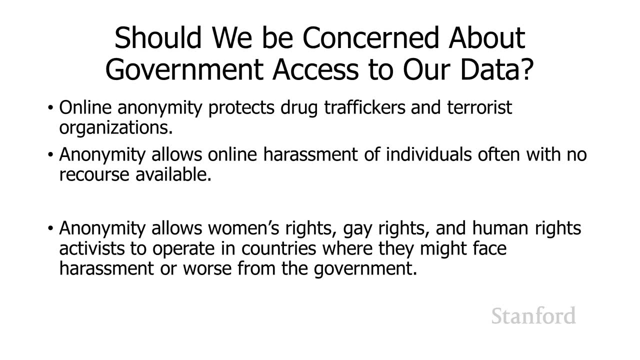 So just be aware of that on the emails I'm sending to you and the emails you're sending to me, All right. so should we be concerned about this? Should I be concerned about the fact that the US government, maybe the NSA, can actually break? 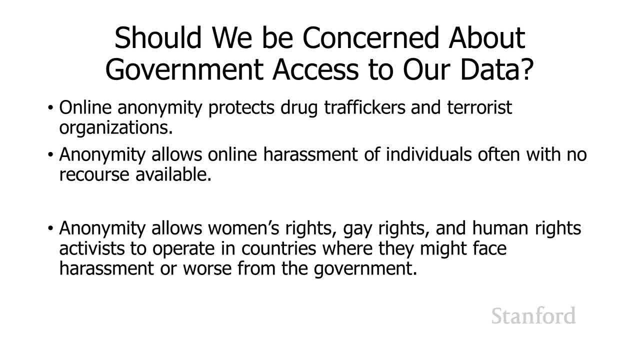 into my account. Well, here's some things to think about. Online anonymity protects drug traffickers and terrorist organizations, and it also allows online harassment of individuals, often with no recourse on their side. On the other hand, anonymity also protects women's rights, gay rights and human rights. 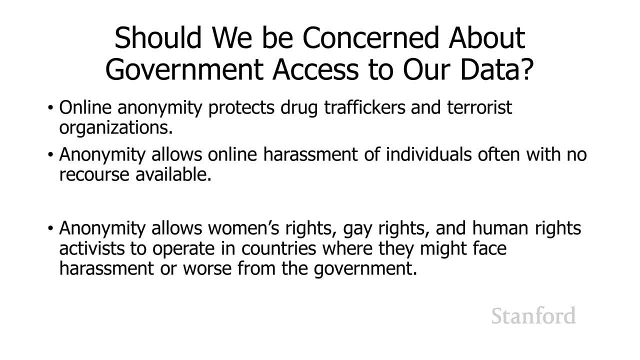 activists that operate in countries where they might face harassment- or worse, from the government. So I think it's a double-edged sword: On the one hand, privacy can be used for really bad things And on the other hand, privacy can be used for really good things. 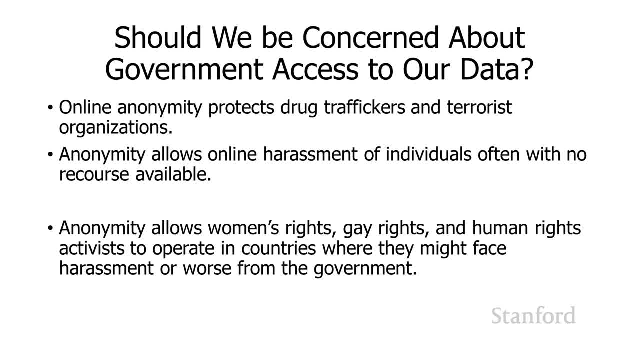 So it's not clear if there's a straight answer on this question, But ultimately, if you want to see what a government can do if it wants to completely track all of its citizens, you can take a look at what's going on in China. 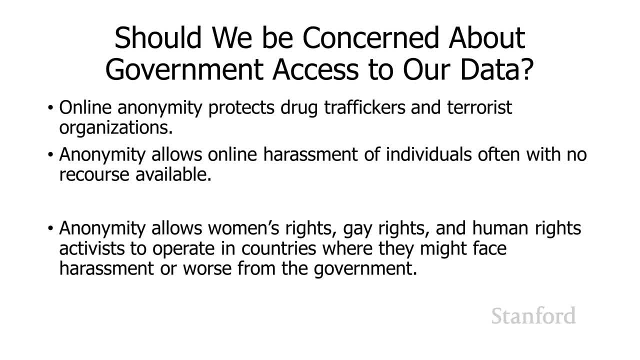 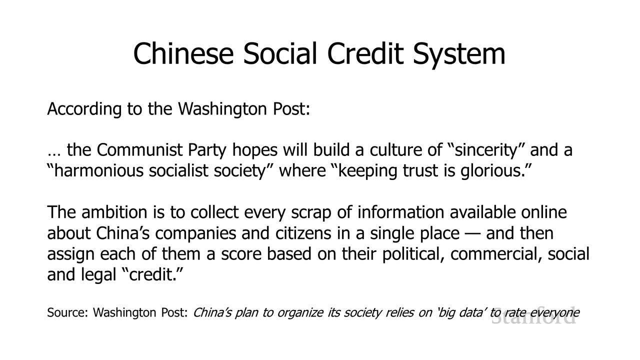 So there's a couple of different things China is doing related to privacy issues, privacy issues and leveraging all of the capabilities of modern computing. So one of the things they're working on is something called the Chinese social credit system. According to the Washington Post, 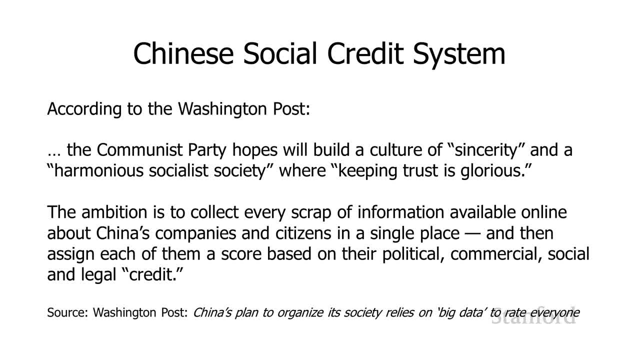 the Communist Party hopes to build a culture of sincerity and a harmonious socialist society where keeping trust is glorious. The ambition is to collect every scrap of information available online about Chinese companies and citizens in a single place And then assign each of them a score. 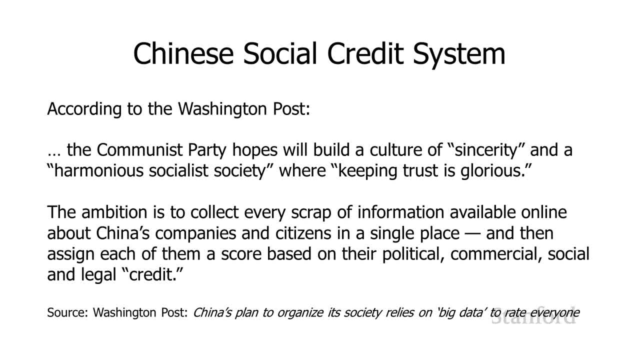 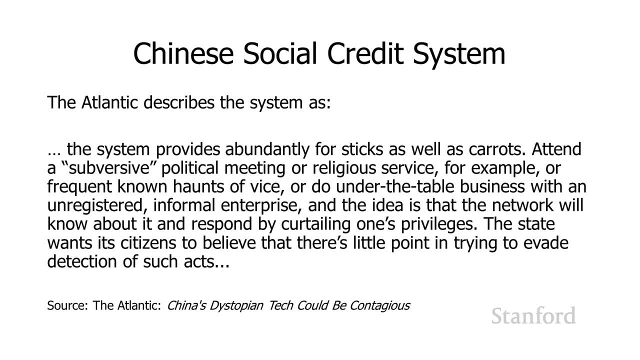 based on their political, commercial, social and legal credit. The Atlantic describes the system as the system provides abundantly for sticks as well as carrots. Attend a subversive political meeting or religious service, for example, or frequent known haunts of vice. 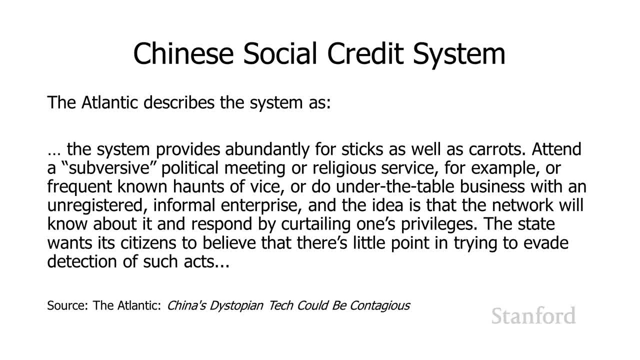 or do under the table business with an unregistered informal enterprise, And the idea is that the network will know about it and respond by curtailing one's privileges. The state wants its citizens to believe that there's little point in trying to evade detection of such acts. 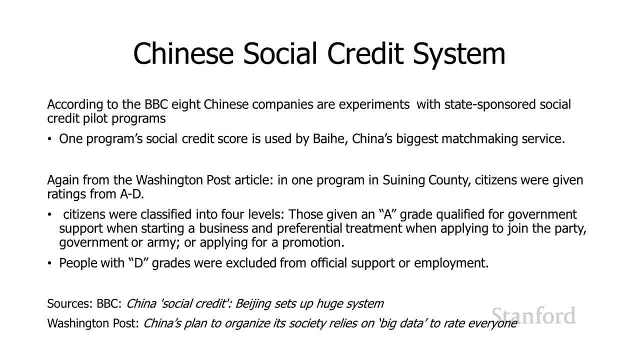 According to the BBC, eight Chinese companies are experimenting with state-sponsored social credit pilot programs. One of the programs, social credit scores, is used by and in spite of having taken Chinese in college for a quarter, I'm afraid I can't pronounce Chinese. 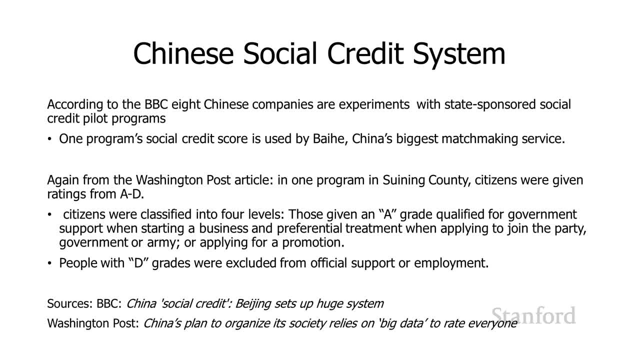 So I'm going to say Baihe, but that could be totally wrong, Sorry guys. Japanese biggest matchmaking service. So the idea here is they're using social credit score for matchmaking. And again quoting from the previous Washington Post article- and there are links to all these articles- 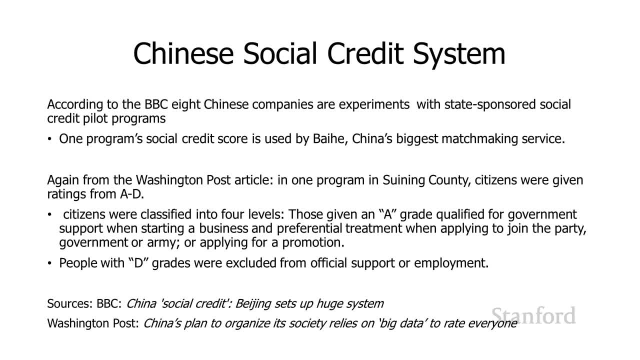 in the class notes. According to the Washington Post, in one program in Swineney County, citizens were given ratings from A to D. Citizens were classified into four levels. those with an A grade qualified for government support when starting a business and preferential treatment. 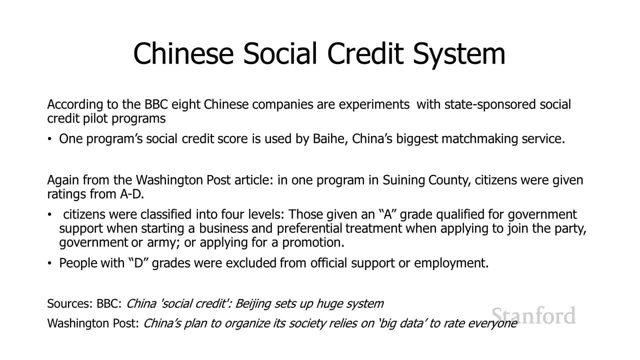 studying and education Academically the ones with a test score. the highest score is at 16.. when applying to join the party, government or army, or applying for a promotion, People with a D grade were excluded from official support or employment. 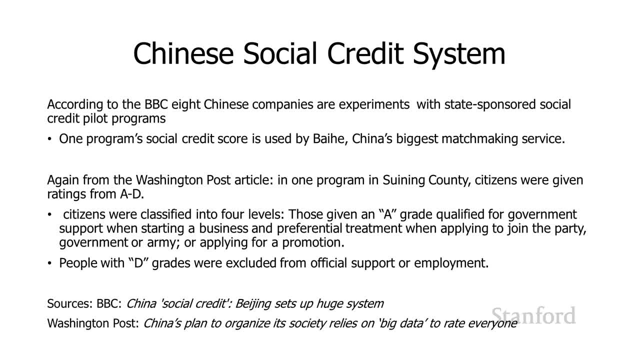 So basically, the Chinese government is taking all that information that we started off this lecture with saying. hey, because we're now in the digital world, it's super easy to track your movements, It's super easy to see what sort of books you're reading. 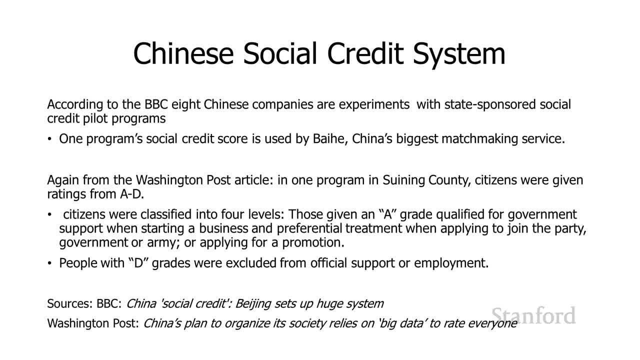 what sort of movies you're watching. They can tell who you're talking to. The Chinese government is taking all that information together and deciding how good of a citizen they think you are and how closely you are at following telling the party line, And on that basis they're going to control your access. 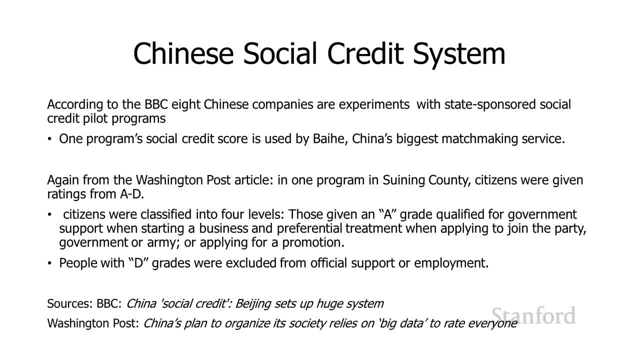 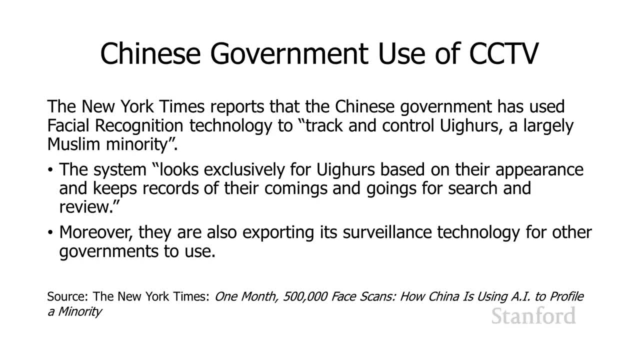 to different resources or they're going to try and punish you if you're stepping out of line. Another thing that they are doing is they're using closed circuit television cameras. The New York Times reports that the Chinese government has used facial recognition technology to track and control Uyghurs, a largely Muslim minority. 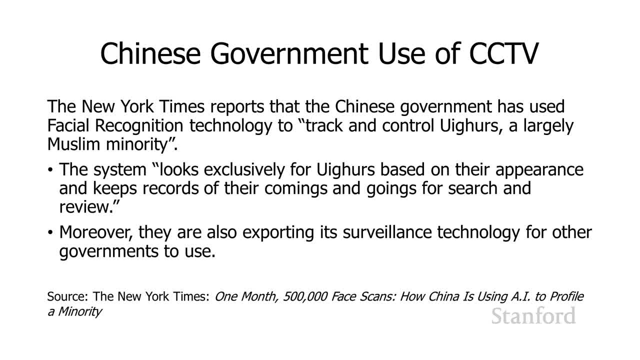 So, if you're not familiar, the Uyghurs are the group that is literally being placed into camps- re-education camps- on the basis of their ethnicity and their religious beliefs. The system looks exclusively for Uyghurs based on their appearance and keeps records. 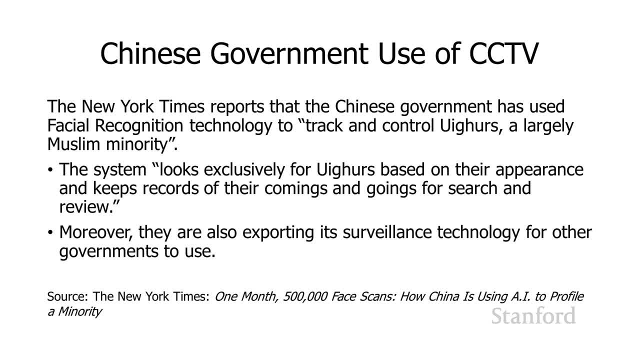 of their comings and goings for search and review. In addition, the Uyghurs are a group of people. The Chinese government is exporting this technology to other governments which are interested in also controlling their population, So I find both of these rather disturbing. 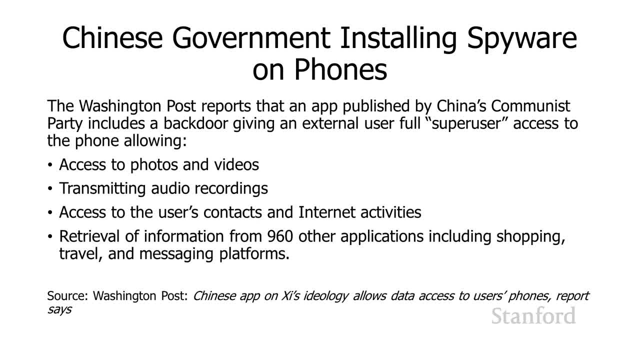 The Chinese government is also working on spyware on cell phones, And so there was an application that was being pushed by the Chinese government, And some researchers went in and basically tried to study what this application was, What this application was actually doing, And they discovered that the app included a backdoor. 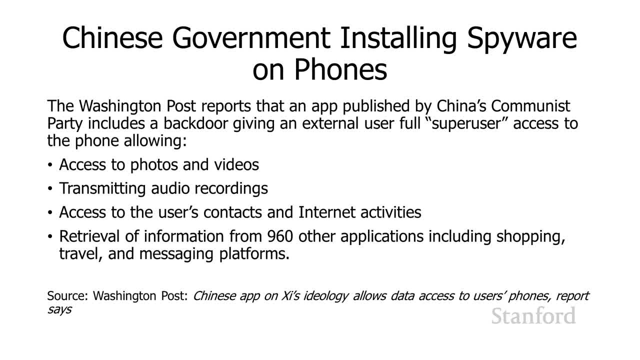 giving an external user full super user access to the phone. Super user is essentially the operating system has different levels of protection, allowing different users different ability to access different things, And super user basically means the top level of user, the one that can do anything they want. 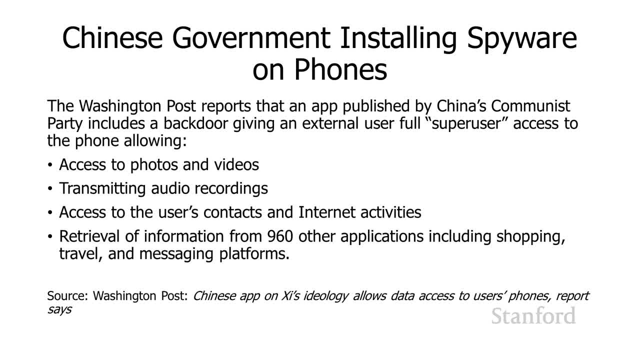 And this level of access allows them to access the photos and videos, audio recordings on the phone, access to the user's contacts and internet activities And, in addition, it's able to retrieve information from 960 other applications, including shopping, travel and messaging platforms. 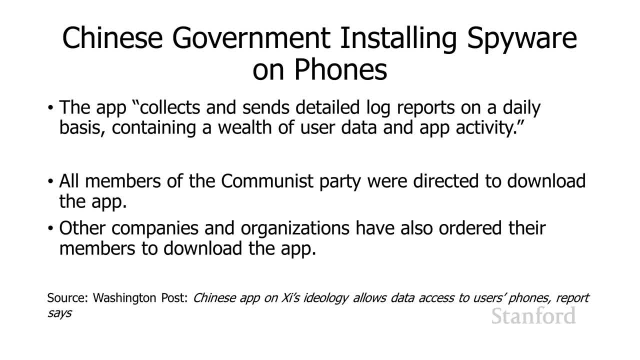 The app collects and sends detailed log reports every day containing a wealth of user data and app activity, And all members of the communist party were directed to download the app As well. the app is able to collect and send detailed log reports As well as other companies and organizations. 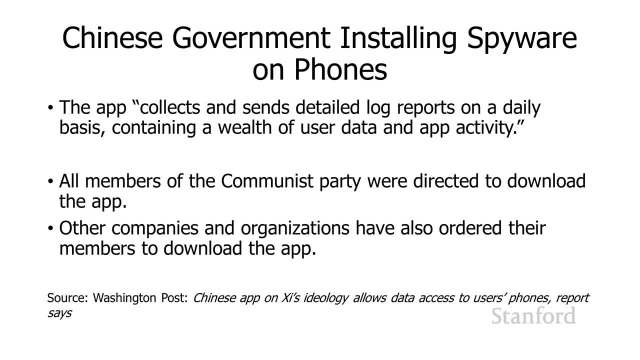 were also pushing their members to download this app. So, bottom line, I think there's potentially a lot of bad things that can happen because of what's going on and how we've moved to the digital world, And I think it behooves us all as citizens. 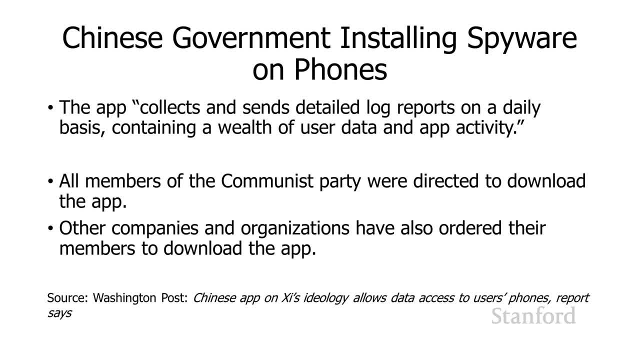 to keep track of what's going on and to try and push our government to limit what both the government and the government do, Both the government itself and what companies can do, Because ultimately, when you move to see what a totalitarian government can do with all this information, it's actually pretty scary.